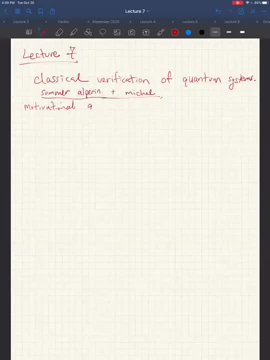 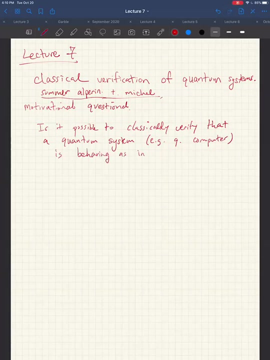 Okay, so back to the. you know the explanation of the section. So the motivational question is: is it possible to classically verify that a quantum system, such as a quantum computer, is behaving as intended? Okay, So there's a number of reasons why we would be interested in this question. 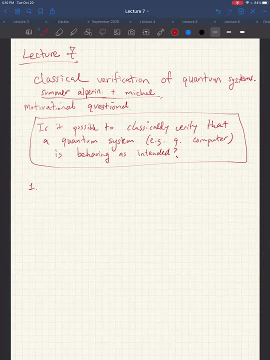 So you know. so here's a little story. So like, imagine that there's a company called Quapple. You know they sell you a QMAC for the cool price of a gazillion dollars. Right, You take it out of the box and you know you run it through its paces. So you know, the first thing that you probably want to try is: okay, can it factor large integers? 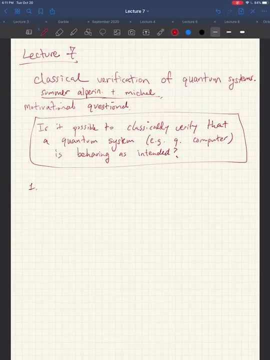 So you know one way to test. this is okay, you pick two primes, P and Q, And you know you ask it, so you multiply the two primes together, you get some large integer N, and then you ask: 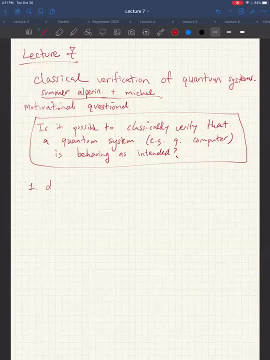 can it actually factor N? And you know the computer will. if it returns P and Q, then you're going to say, okay, well, it seems to be doing a pretty good job. So you know, for those types of problems, like for problems like factoring, you can easily check if it's doing the right thing, right, So, for example, can verify. 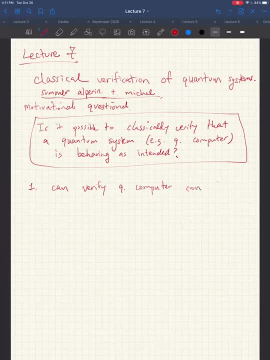 a quantum computer can factor. right, That's so. that's one thing you can do for verification. But what if you want to solve some other problem, like you want to simulate the evolution of a Hamiltonian Right. So let's say you have a local Hamiltonian H right Describes your, you know some physical system of interest And what you'd like to do is say, well, I'd like to evolve this Hamiltonian. So you, there's this operator E to the minus N right, And you can do that. 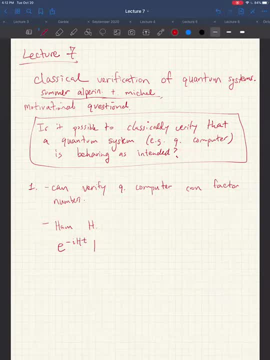 This is a unitary operator and you want to apply it to some initial state. Let's say it's like the all zero state or something right. You want to. you want to evolve this Hamiltonian. This is something that you can do in polynomial time. 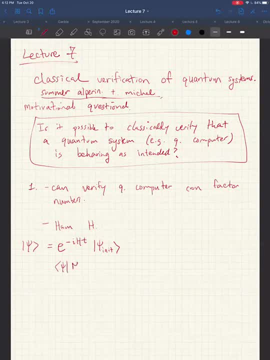 And you want to say: given the results of this evolution, I want to estimate some observable M on the state. So this is what you want to calculate And this is basically like what you know quantum computers were meant to do: to solve problems. 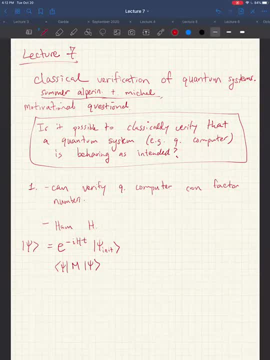 So you, you know, you program up this, this cube Mac, you know, using your favorite Hamiltonian simulation algorithm that's in the literature, And you run it and it spits out some number. Let's say it spits out 42. Okay. 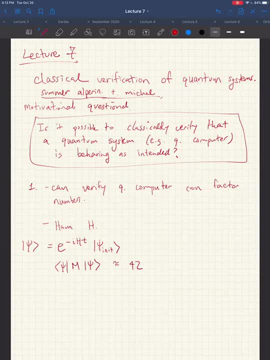 How do you know whether this is actually the correct answer? Right, First you have to check whether you asked the right question. Right, Exactly, So exactly, You know. so let's say you even figured out whether you asked the right question. 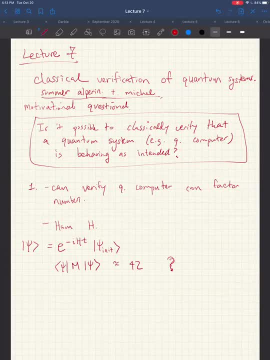 And conditioned on that, then you want to know if this is the right answer, And this is not so obvious- how to do right Because, like the whole point of buying this, you know quantum computer is it was supposed to. you know this task was supposed to be intractable for, for classical computers. 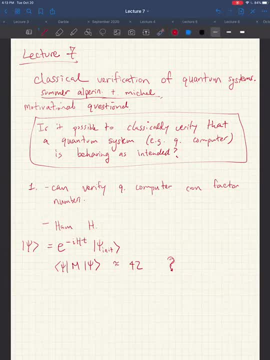 Right Like it, you know it. presumably, in general, it should take a classical computer exponential time to figure this out. So so how would you possibly know whether the quantum computer was doing the right thing? So so that's one reason why it's an. you know, it's an interesting and important question to come up with classical verification schemes for for these. 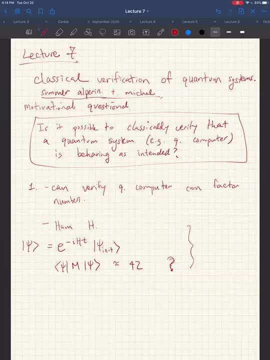 These types of quantum Computations, And it's not, you know, just about being paranoid. Right Like today, people are trying to build quantum computers And you know the quantum computers are trying their best, but they're very noisy and they're very primitive. so you'd like to have some assurance or some certificate that whatever answer that these computers are giving you, it's, it's not due to noise, It's not just some noisy junk output, but it's actually something accurate. 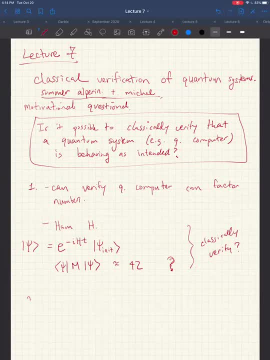 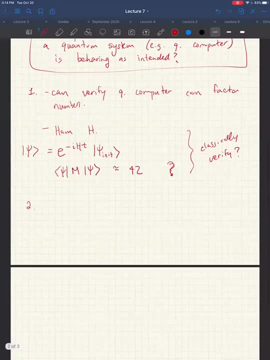 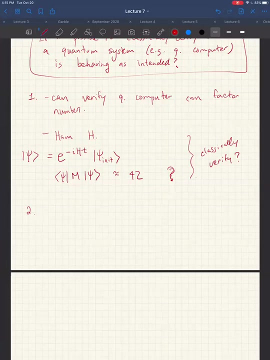 Right, So. so that's like a practical motivation. There's, there's another motivation which is like to me, maybe actually more interesting, which is a little more philosophical, Which is that, You know, quantum computers are not just bigger and faster versions of classical computers. they're, they're, they're actually qualitatively different than classical computers. 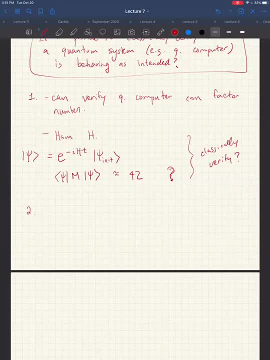 You know, one way That they're qualitatively different is that our best attempts at trying to come up with a classical description of what's going on inside of a quantum computer would require exponential resources. right, and it's really unlike anything that we've built or designed before. um and so, given that it's so, 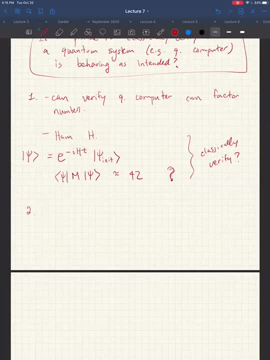 different and from you know, anything that we're used to. um, it seems like it really just it justifies, like, additional skepticism or scrutiny on whether these fantastic machines that you're building could, could actually be ever be made to work. um, you know, and there's also a lot of skepticism. 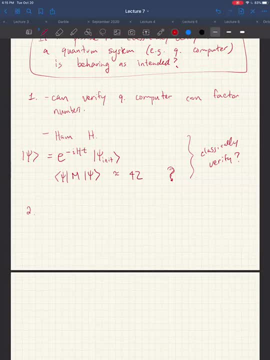 out there whether quantum computers are possible at all. um, and some skepticism is more scientific than others. uh, so, for example, there's a famous mathematician, um you know who's maybe at the of quantum computing. skepticism, um, you know. so there's this guy named Gil Kalai. 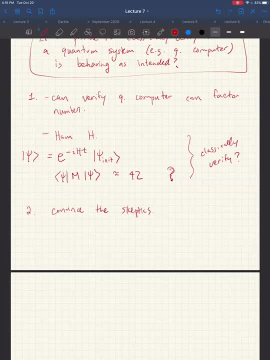 and you know they, they're very um, publicly uh um. or you know they, they have proposals for why quantum computers cannot work in principle, um. and, for example, Gil Kalai's main argument is that once you scale up your quantum computer, you're going to be able to do a lot of things. 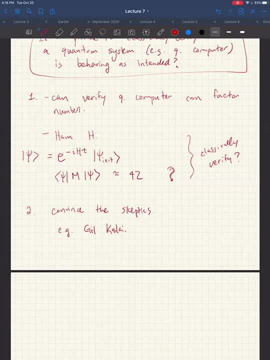 um, but if you scale up your quantum computers beyond a certain size, um, there'll just be these, um, these correlated errors that actually prevent your system from, uh, from doing anything that cannot be classically simulated, or you know, just to say it more simply, you know the errors will. 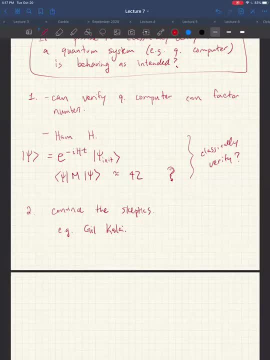 accumulate in such a way that whatever's happening in your quantum computer it can be classically simulated. so you cannot achieve a um. you know this, this quantum speed up um. so you know it's not clear how much water his proposal holds. there's, uh, you know it's it's. you know he doesn't come out with. 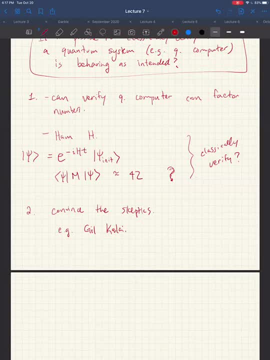 like a very precise model that can be refuted, proved or disproved, um, but you know it's a serious attempt at trying to poke holes, at at whether, um, quantum computers uh, can work at a large scale and um, so it's worth, you know, trying to meet the skepticism head-on and trying to come up with 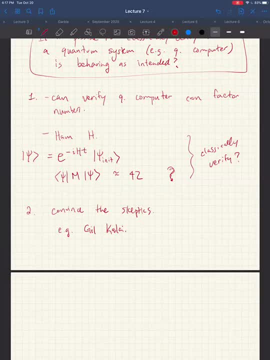 very principled and sound ways to to try to refute their arguments, right, um, you know there's this henry. yeah, has he, as he said, as the? this guy said anything about the supremacy experiment? oh, he said a lot of things about the supremacy experiment. um, there's, um, he's given a bunch of 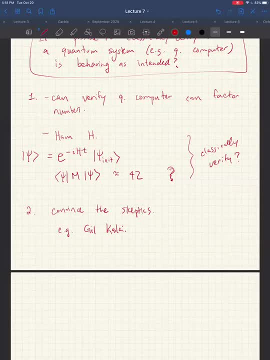 talks and uh, you know, unfortunately i haven't watched them in detail, but i think um he actually he raises some good points. at least in the stuff that i've seen, he says that the? um. so in these, like for example, the google's quantum supremacy experiment, they have some statistical 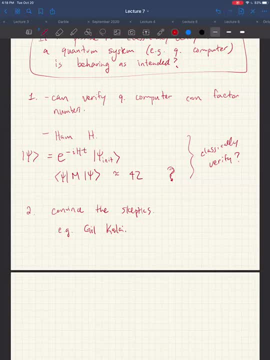 verification for for why they think that the google's device actually passes this. you know this supremacy test, um, but they actually- you know the google folks- used a bunch of heuristics and um assumptions, for example, about the types of noise that that, uh, you see in the system, um, and i think 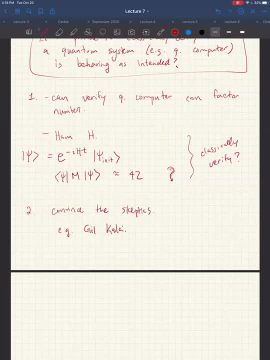 what gil khali is saying is that, um, that this assessment of the noise is too simplistic and it still leaves open the room, that actually it's. um, you know that that it's it's not working, as well as, say, the, the google folks think it is. 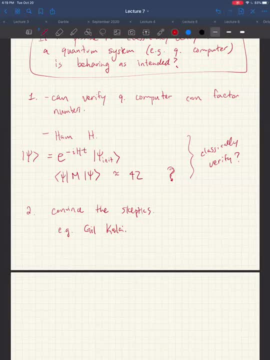 um. now what? at least my opinion is that i think, uh, i do agree that the, the google's noise model is too simplistic, but not in this damaging way that that gil khali believes in that. it is um, so that's, you know, that's my opinion, at any rate. i think he even wrote a paper on that. 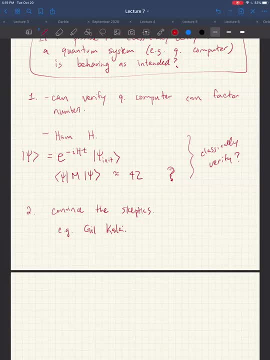 specific uh experiment called the statistical aspects of quantum supremacy demonstration. for some reason i cannot live here. maybe you can look it up. oh, yeah, uh. so if someone can find the link in the description, i'll put it in the description and i'll put it in the description. 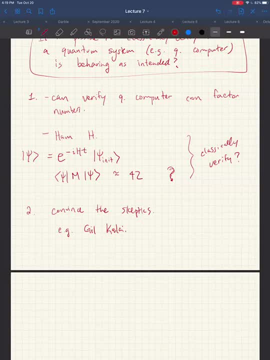 and maybe post it in the chat or in the slack. that that would be great. so people are curious, so he's come out. i mean he's. he's had this skepticism for many years, um, and his arguments have evolved, but i think it's a very useful um. 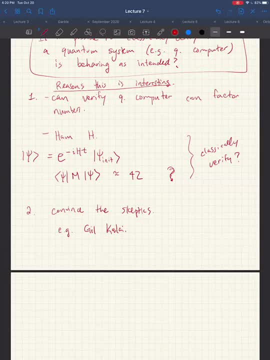 it's useful for the science. because you know you need people to at least credible people, and i think gil khali is um very credible because he's he's a professional scientist, he's a mathematician that's very accomplished um and you need them to to push back on on um on you know our claims that 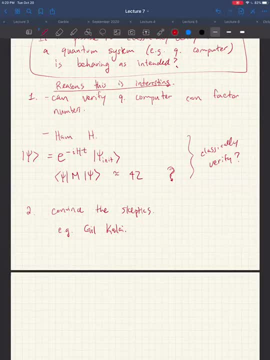 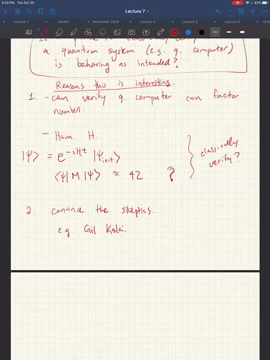 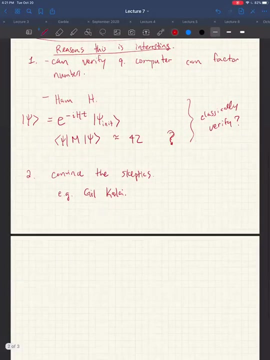 so, um, i think if we developed, you know, means or methods or protocols to verify whether a quantum computer is working correctly, without assuming that, without assuming that you have a quantum computer to begin with, that that would be a great way of answering this challenge. um, so that's, you know, kind of, uh what, you know the motivation behind um this, uh. so so what are? 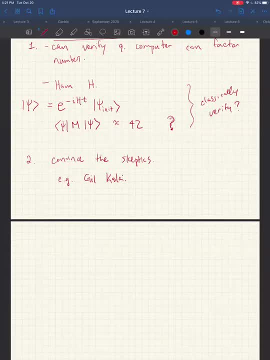 we going to talk about in the next six weeks of the class? um, well, there's been a lot of progress, both theoretical and experimental, on methods for verifying quantum systems, um, and we're actually going to cover the more theoretical angle, um, so, uh, we're going to talk about. um, one thing we're going to talk about is, uh, a specific 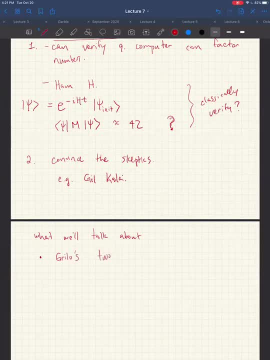 protocol that's due to alex grillo. so alex grillo has a two prover protocol for verifying quantum computations. all right, so so this is a in this setup in his protocol. basically, we have a classical referee, you know, imagine that it's a classical skeptic um, and they want to run a quantum computation and they interact with, you know, not one quantum. 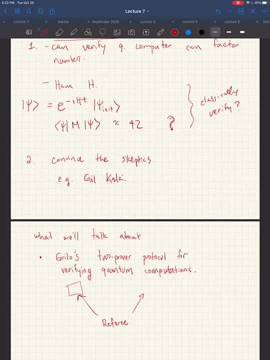 computer but say two quantum computers that are separated right, and this should start, look to start, look a little familiar to stuff we've seen before. and, um, the referee will interact with these two quantum computers, uh, classically, just sending you know, classical messages back and forth, and at the end the referee should be able to uh to verify whether the 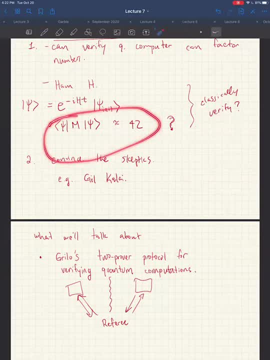 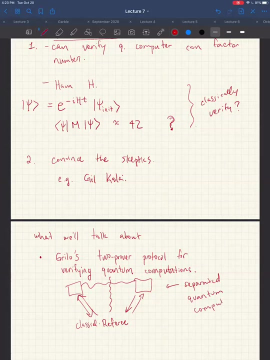 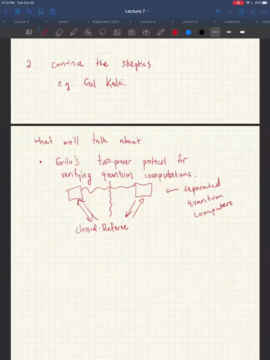 the result of say, for example, this computation really is approximately 42, with high probability. the requirements of these two quantum computers is that they're entangled, that they share quantum entanglement right, and so you can see that you can actually do something like this. so that's one protocol that we'll see and building on on ideas that go into this. 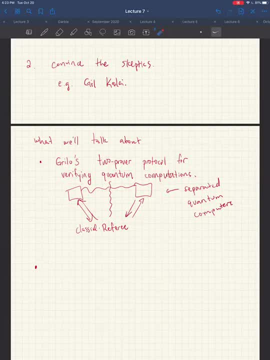 type of protocol where you're trying to verify that these two separated machines are doing something correctly. we can actually um prove results that are actually- uh, they're interesting, not because they related to quantum computation per se, but because they have. they have consequences for things like complexity theory. 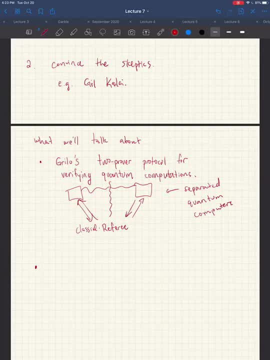 and also pure mathematics. So there's a second result that we'll talk about that's called MIP, star equals RE. This is a complexity result and it has applications to pure mathematics and also mathematical physics And what goes into this results are basically ideas from verification. 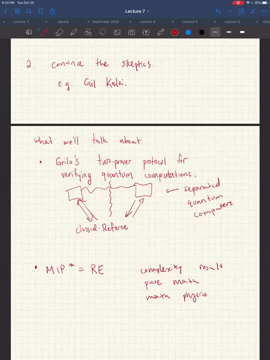 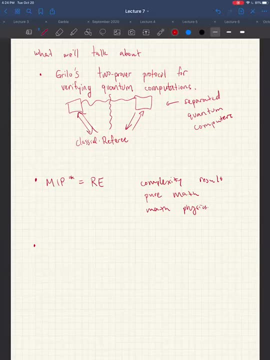 It's really central to this result, And so we'll talk about that in a couple of weeks And, if we have time, then we'll talk about another protocol. but it's slightly different characters, So at this time it's a single prover protocol. 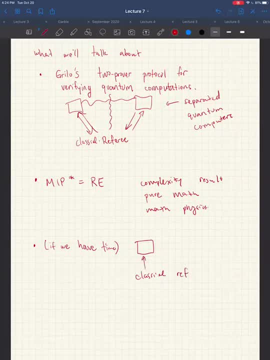 So it's: you have a classical referee and it interacts with only one quantum computer. So you don't need these two quantum computers anymore And you can verify that this quantum computer is correct. So this is a protocol due to MahaDev. 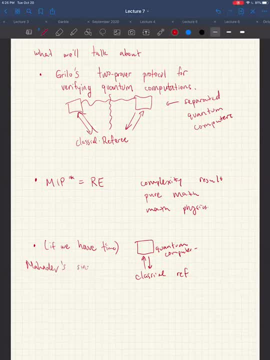 So it's, you know, it just takes a little bit of time and you just keep on going. It's a lot easier than using the, And what's interesting about it is that, in order to reduce the number of provers or quantum computers you have to interact with in order to do this verification. 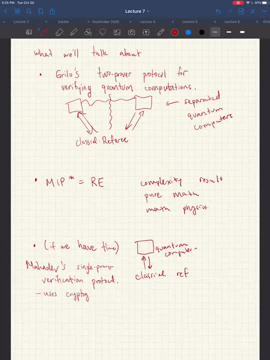 you make use of cryptography. the cryptography is a way to sort of force this, you know, quantum computer to do what, what you want it to do, in in some verifiable way. ask a question, yeah, um, with regards to the two prover protocol, um, like i don't understand why we want them to share entanglement to me, 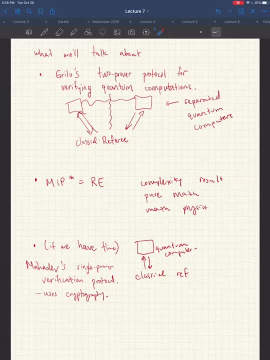 it would seem, you know, more impressive if the computers are, you know, easier to verify and more impressive if they could do it without that entanglement. and furthermore, um, once they're sharing entanglement, i'm not really seeing in what sense they're two quantum computers to me. 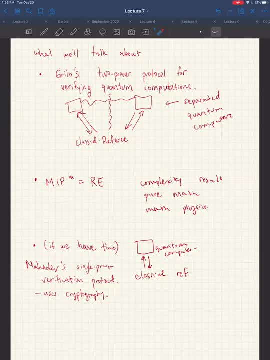 they seem very similar to one quantum computer. okay, good question. so that's right, i mean, it would. it would be, um, uh, if you could do it without them sharing entanglement, that would, yeah, that would be great. i mean also, that would tech, you know, in terms of practical concerns, it would make it. 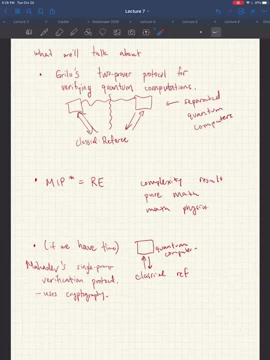 easier to implement this protocol. right, it's, it's. the entanglement is actually um needed because without it, the, the, these two quantum computers, couldn't coordinate their responses in a way that would convince you that they were doing the right thing. but doesn't it also allow them to, you know, coordinate? some clever way of fooling me. 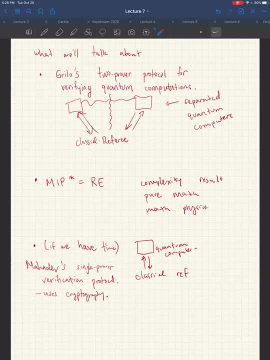 and i guess that's you know once, once we see the actually actual protocol, we'll have to address that concern exactly. so that definitely is something you have to uh worry about, um, but it turns out that the protocol will will have these checks to ensure that they aren't um. and for your second question: um, why is? 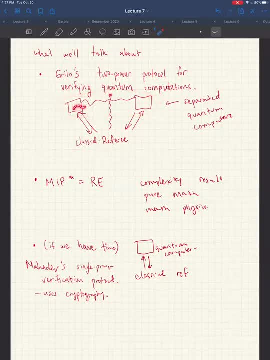 two different from one? well, um, they're. they do share entanglement, but they're still not allowed to um communicate and in the sense that this computer right here does not see what you're asking the the other computer, because entanglement doesn't allow you to, you know, communicate and this constraint is um very useful. 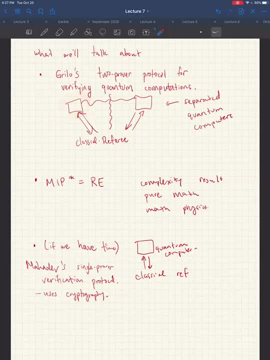 so basically you can, you can um, enforce that the uh. you know in some sense that their behavior is is honest. it'll become more clear when we get like explain how the protocol works, but those are really good questions. yeah, so maybe another uh kind of silly question: if they don't share quantum uh entanglement, then this basically: 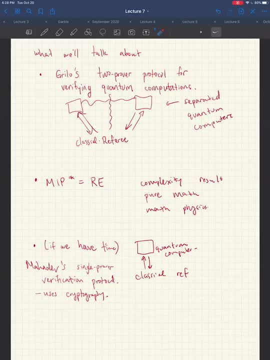 boils down to m to mip without a star right and they can choose to not share entanglement right, like it's up to them right, and so like, how can you beat next if they can choose to never allow? allow you to beat next by just not share, share anything. 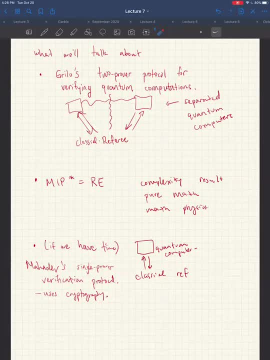 um, well, uh, let's see. so i didn't quite get that, but well, i mean, i sort of get what you're saying, so, um, so there's a. there's one important thing that i want to emphasize is that this, in this protocol, these two quantum computers are assumed to be quantum polynomial time. so it's, it's actually. 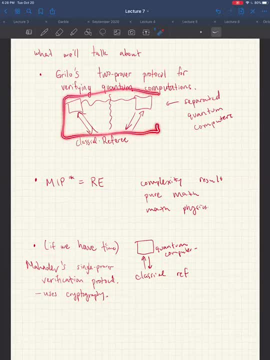 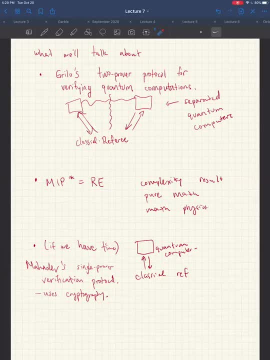 but there the provers were allowed to be infinitely powerful, here we actually, because we want this to be, you know, potentially a real world, applicable protocol. so the the demands on the these two quantum computers is they should be able to, um, to run this protocol, uh, in polynomial time. 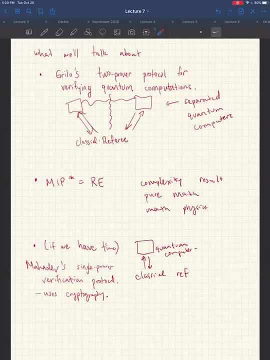 oh so, so in, in particular, they won't be able- we don't expect them to be able- to solve- uh, you know, uh annex complete problems. so that's okay. yeah, does that? does that answer your question like that? that illustrates some difference between the two complexity classes that i can assume will lead to some implication that i'm 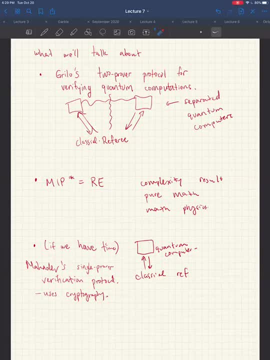 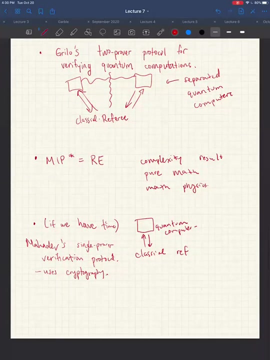 not yet yet seen. Yeah, The point is that this entire protocol can be simulated in quantum polynomial time, So cool, Yeah. Any other questions about sort of the setup or the theme or anything like that? Okay, So this is where we're going, So let's dive into it. So the key workhorse behind 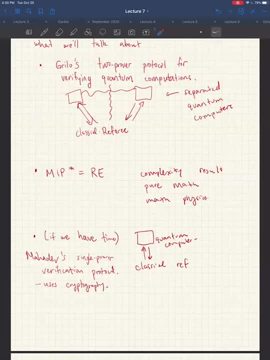 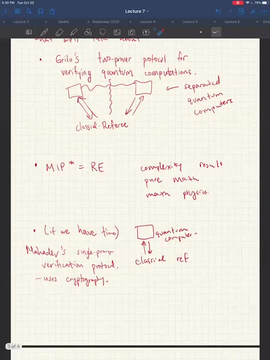 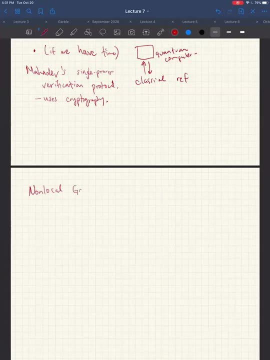 these two results is going back to something we covered in the very first lecture, which is the CHSH game. Right, So you know. more broadly, we're going to talk about how non-local games can be used for entanglement testing And really the way we should. you know, you should think. 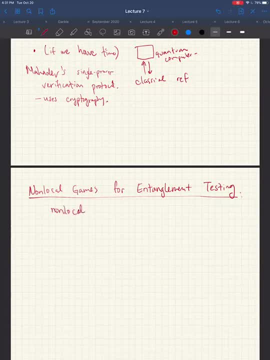 about this is that non-local games, of which the CHSH game is is like the primary example, is a way to like force quantum systems to do what you want them to do in a class, like you can classically force them to do. 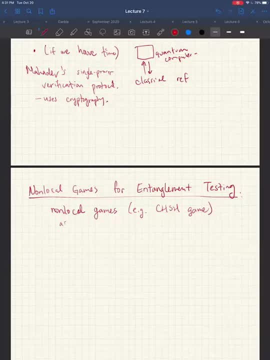 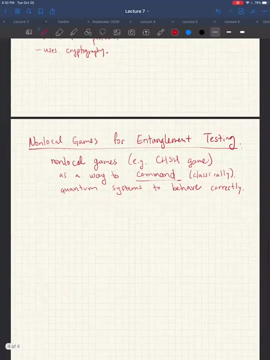 specific operations. Okay, Okay, All right, So. so let's recall the CHSH game. All right, So I'm going to be drawing lots of these. pick, you know these. let's see, I'll pick this one up, So I'm going to pick. 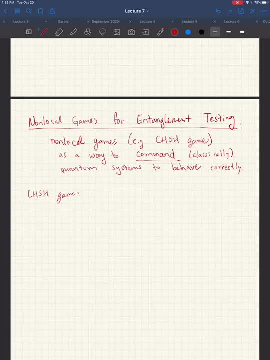 this one up these two prover pictures for the remainder of the class. So we have two players, let's. you know we call them Alice and Bob, And you know there's a referee. The referee will choose a random bit. 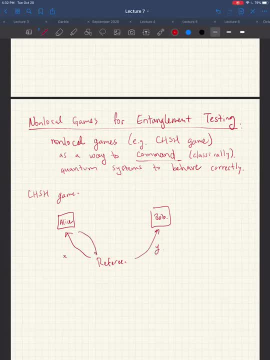 send it to Alice. choose a random bit Y send it to Bob. They respond with bits A and B and they win if the sum of their answer bits is equal to the product of their question bits mod two And if Alice and Bob are classical. 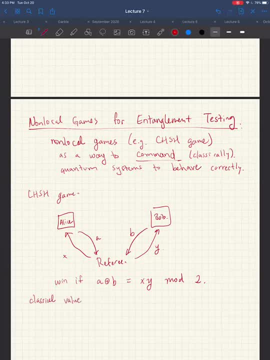 they use a classical strategy, then the classical value of the CHSH game, and I'll denote that by omega, which will look a lot like W. but omega of CHSH is equal to three quarters. But you know, we saw in lecture. 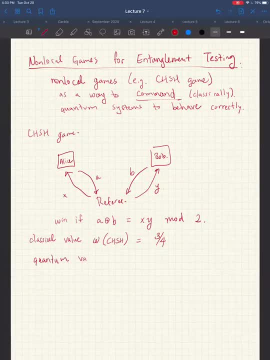 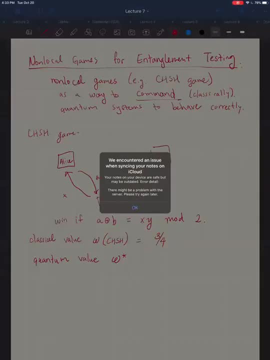 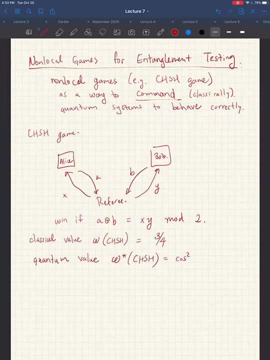 that if Alice and Bob share quantum entanglement, then the quantum value which I'll denote using omega star- the star just means like they're allowed to use. okay. quantum entanglement is a larger quantity. It's this cosine squared pi over. 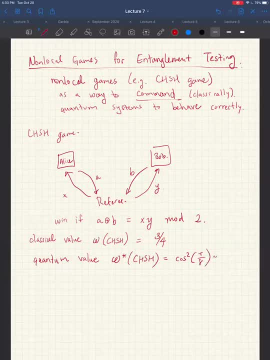 or eight, was it? Yeah, power eight, which is, you know, .854, dot dot, dot. Right, You know, and you know the strategy, the quantum strategy that they can use to obtain this higher value. is pretty simple. 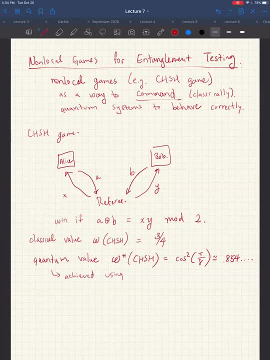 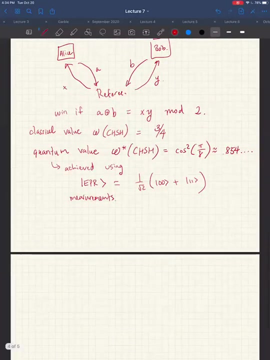 This is achieved using, you know, EPR pair shared between Alice and Bob. Okay, So it's this simple two qubit entangled state, maximally entangled state, and their measurements. you know we can describe their measurements in terms of these binary observables, right? 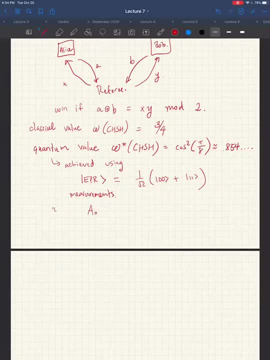 So if Alice gets question X equals to zero, then she measures this observable which corresponds to the poly Z observable Right. If she gets X equals to one, then she measures the X observable right Or she measures in the X basis. 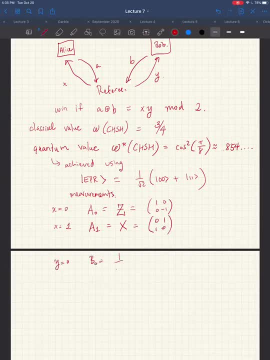 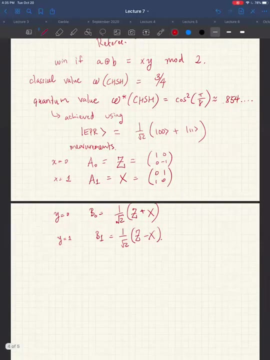 And for Bob, his strategy is some linear combination of these, And so it's a pretty simple to describe strategy, and using the same formula, you can get the same result. Okay, Using this, they can achieve this quantum value 0.854.. 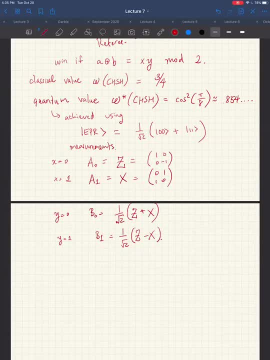 All right, And you know the reason we were talking about the CHSH game to begin with is because we were thinking about this. you know this: Bell test right, Bell's theorem. Bell's theorem was saying there cannot be a local classical theory. 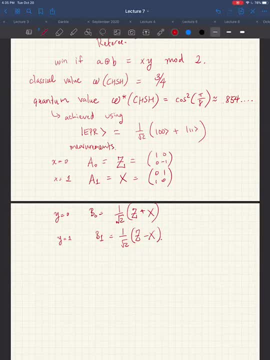 that reproduces all of the consequences. predictions of quantum mechanics. What if if there was aoretically got dusty CIK, How Och letzte, And you know concretely How Och MAX talvez. Well, if just to see, 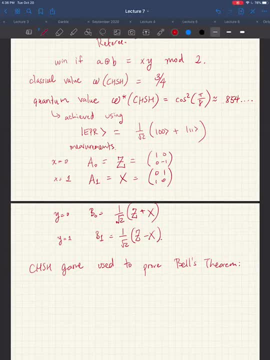 well, suppose that you ran an experiment. What's great is, if you want to take the cell, you played the volt-c Sciatica H shame with two players, Alice and Bob, what you can do- And you see that they're winning with higher than three-quarters probability. 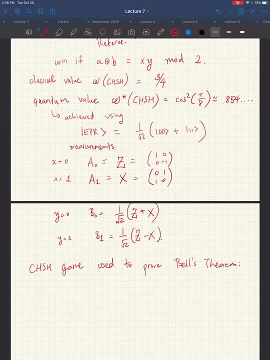 then what you're forced to be able to do is simply mathematical. the steps you now have in front of you Nevada to believe is that they're using some kind of quantum entanglement in their strategy. They cannot be using a classical strategy. 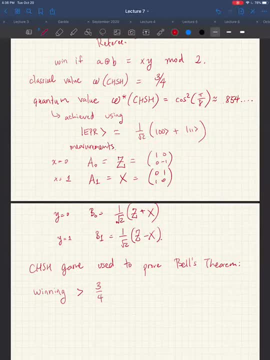 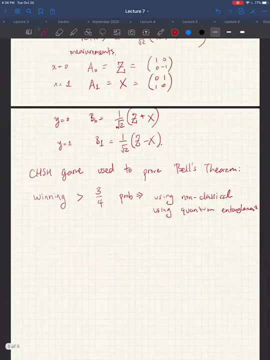 So if you're running strictly more than three quarters of the time, is that you're using some, doing something non-classical. in particular, you're using a quantum entanglement And it's sort of a way to like at least verify. 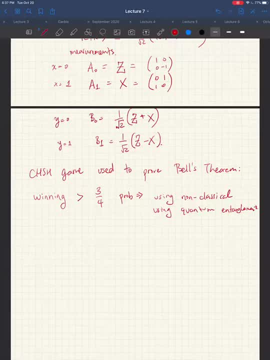 that nature is behaving non-classically. So that's pretty cool, But we're actually gonna go further now, because the CHSH game actually tells you a lot more, If you're suppose that they're winning not just greater than three quarters of the time, but very, very close. 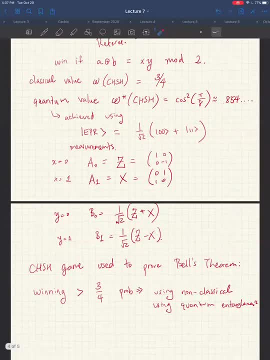 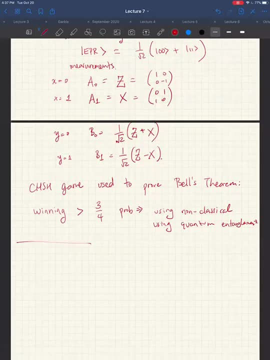 to this quantum value of 0.854, then in fact, you know that they must be using a specific type of quantum strategy And because of this we say that the CHSH game has rigidity or we say that the CHSH game is rigid. 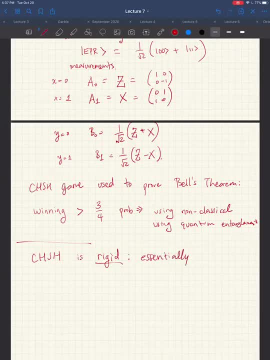 Essentially, there's only a unique way, There's only one way to win the game close to optimally. Is that one way like given that quantum mechanics is correct, or like one logical, theoretically possible way? Great question. Well, assuming quantum mechanics is correct, 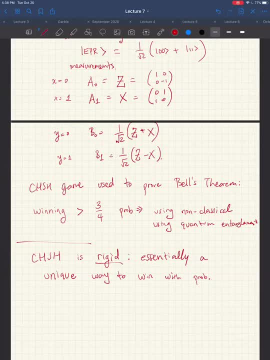 like assuming that the way that the players are described is using quantum theory. then there's essentially, you know, describe what essentially means, but essentially one way to do it: quantum mechanically. So, yeah, good point, So within the framework of quantum mechanics. 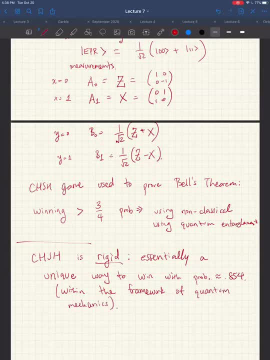 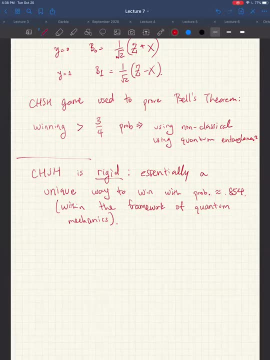 But I guess that this requires a proof, right, Like who knows if there's some weird proof, right, Or some weird protocol out there that achieves the same winning probability? Yes, And basically the rest of the lecture is going to be devoted to this proof. 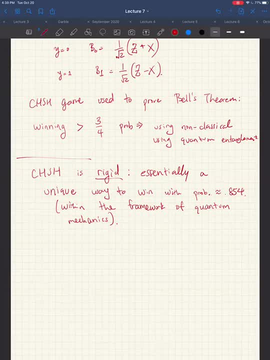 So we're gonna see why the CHSH game is rigid And, just to you know, prime you. this rigidity will be the thing that allows us to do this, this verification, because you know, suppose you play the CHSH game like in the beginning. 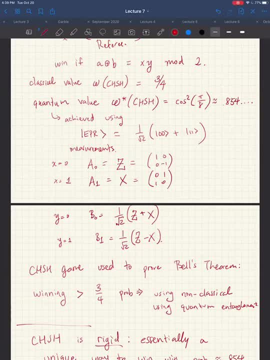 you know Alice and Bob. they're completely uncharacterized. They may be like extraordinarily complicated that you know who using who knows what kind of quantum state, what kind of quantum measurements, but by playing the CHSH game if you can somehow determine that they're actually just. 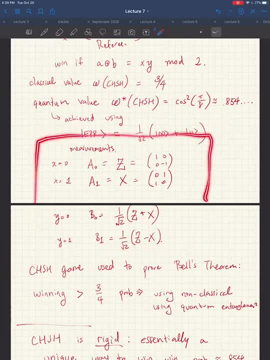 doing this. you know that's a very powerful kind of characterization And just by and once you have, you know, this gets your foot in the door. then you can start playing a bunch of different CHSH games together, in some, you know, orchestrated. 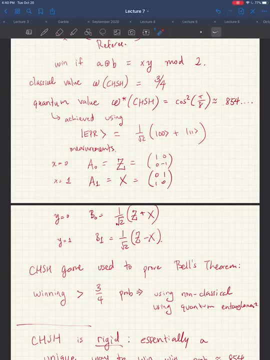 carefully put together way And then you kind of: this is how you start commanding them to do: you do this operation, you do this operation and then you control them to do arbitrary quantum computations, just starting from the CHSH game. I'm not gonnagendeck you to the speaker for this. 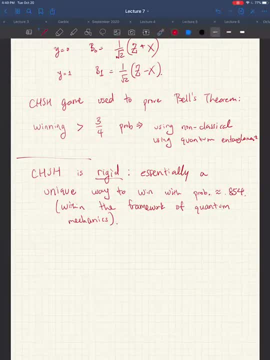 but it's pretty cool. It's not the same as the. I mean It's it still is a little Today's Thinker. I mean, there's so many ways to do this, so I just think it's really cool. 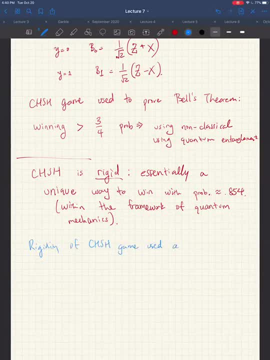 I'll save that for later. Okay, so we can move on to the next one here. Alright, So I'm just gonna show you guys a couple of options that we've made for this course, for the game. So here I'm just going to show you guys. 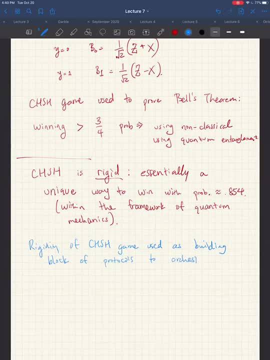 some of the things that we've made for the entire course. You're gonna see all the different software features that we've made for this course. I'm gonna take a look at my dashboard and see how it's done, And so. so that's the why this is super powerful. 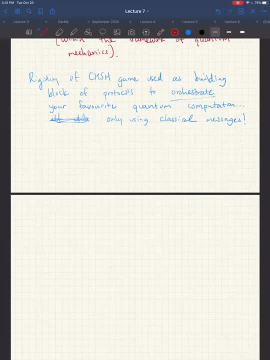 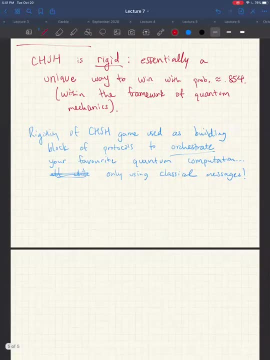 All right. so let's prove it. Let's see how we can actually prove rigidity of the CHSH game. So let's just start all the way. at the beginning, There's Alice and Bob in front of you And you just know that they're described. 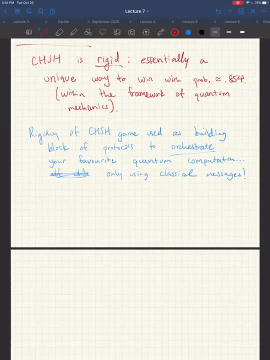 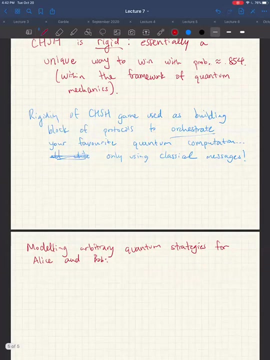 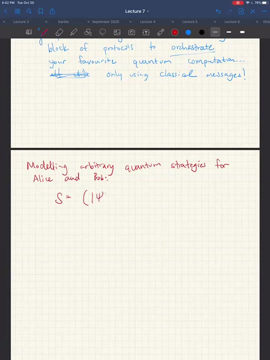 using quantum mechanics. So we have to have a way of modeling arbitrary quantum strategies. All right, so what's a strategy? Well, we can abstractly define it. It's a triple. So you know, you have to say what state they're using. 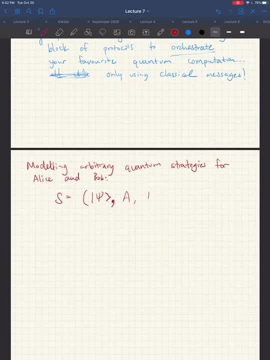 between Alice and Bob And their choices of measurements, right, So this state is some bipartite state, some entangled state in CD tensor, CD okay, For we don't have any control over what this dimension is. Right, so we just know it's a natural number. 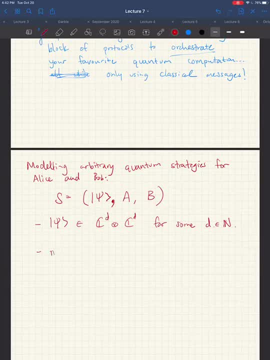 And a choice of measurements. So right, So you know. we know that they're performing measurements depending on their question on this D dimensional state. So they'll choose D by D matrices, AX zero, AX one. These are projectors that sum to the identity. 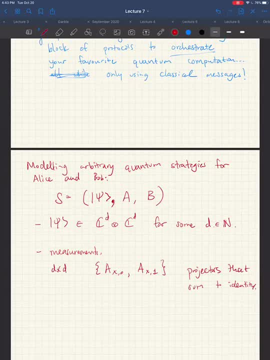 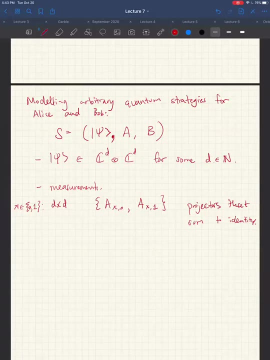 Right, And you know for both choices of X. Sorry, Henry, Is it important that Alice and Bob have the same number of qubits? It's not important, I guess you can always sort of assume, like, let's say, one person had one more. 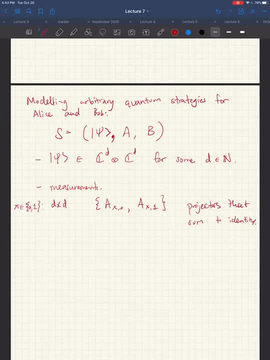 had more qubits than the other. You can always just pad the other person's state with like zeros and they just ignore it. So it's. It's just a little more convenient to say that they have the same dimensions on their side, but it's not so important. 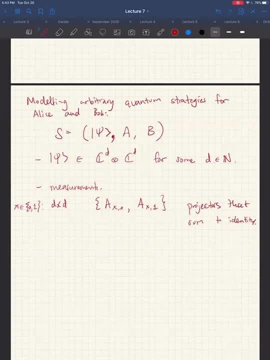 Okay, great thanks And go for it. Does that imply that increasing the dimensionality of one system would never proffer any advantage? We'll see that. yes, For this specific game And actually in general. yeah, in general it actually won't matter. What really matters is not the local dimension on each side, but really the amount of entanglement between the two sides. That's really the important quantity. 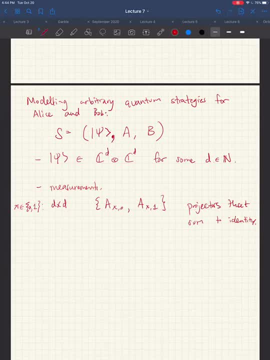 Yeah, You know, just so, like, if this makes sense to you, then great. If not, what matters is just the Schmidt rank of the state that's used between them, And you know so. Alice chooses for both her questions a projective measurement, and so does Bob, So we'll just call it. 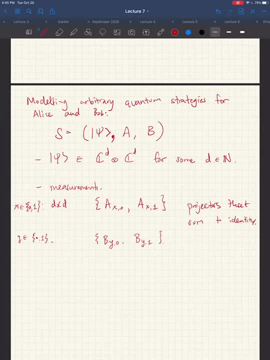 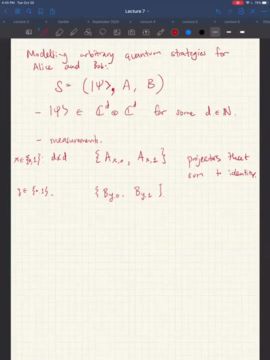 So the you know, the first subscript indicates the question and the subscript, the second subscript indicates the answer. And you know, rather than keeping track of all these different projectors, since they have binary outcomes, we'll just package them into an observable, just because they'll be mathematically nicer. 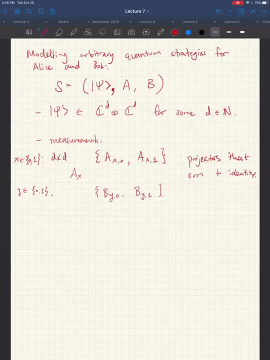 So I'll say that a sub x is the observable a sub x zero minus a sub x one. b sub y is equal to b sub y zero minus b sub y one, And notice that these are observable, so they're actually unitary. 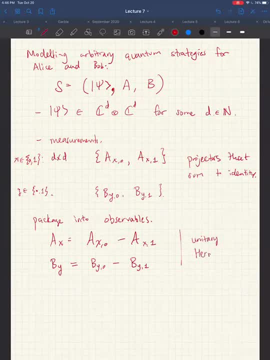 And her mission. So, and you know, another convenient thing about them is that they square to the identity, Like if you, if you square them, it's going to be the identity matrix, Right. So so we'll just work with observables, because it'll be easier and nicer. 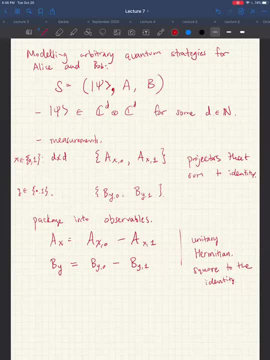 So so that's what a strategy is. You choose a state, you choose your observables, and that tells you everything about how they'll behave in the game. So if someone chooses a strategy like that, then we can define their how well this strategy succeeds in the CHSH game. 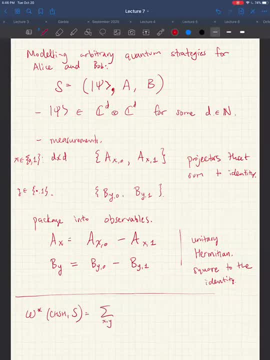 Right, So this will be defined as well. you, you pick questions x and y, with a certain probability, which in this case will be one fourth, You sum over all possible winning answers for, for the that choice of, for those, those questions. 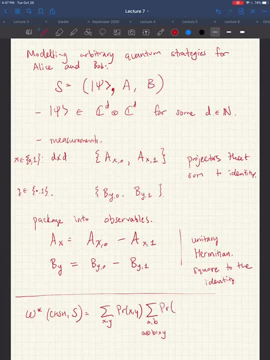 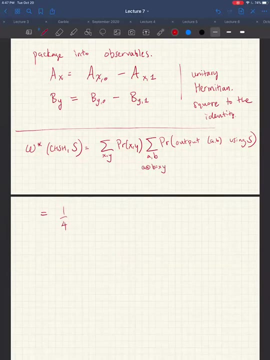 And and then you you look at, well, what's the probability. using the strategy, They output a, b, Right. So I'm just writing out what the definition of what the success probability is And sort of plugging in the right numbers. we get sum over x, y, a, b, such that a plus b equals x times y. 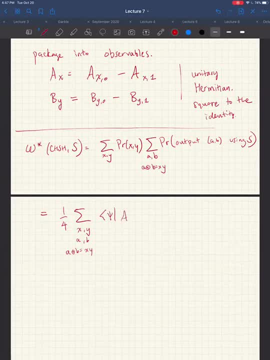 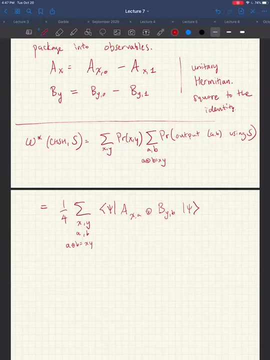 And their success probability is. is exactly this. Just writing out the definition of. you know what's the probability. they measure a and b given x and y. But you know this is still written in terms of projectors and I don't want to write it in terms of projectors. 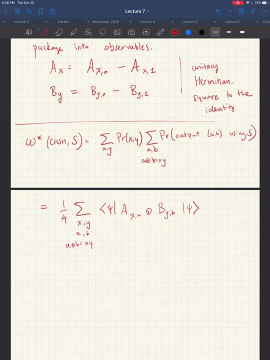 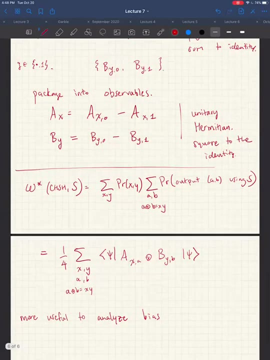 So I'll write it a slightly different way. What's phi here, The state there? Oh, this, this psi. Yeah, psi It's the state that they chose. So it's this bipartite state, right here. 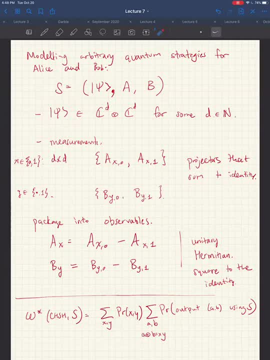 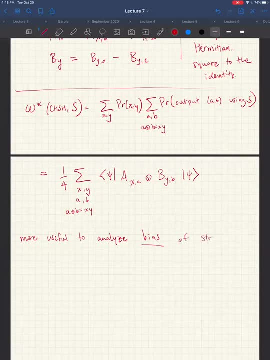 Oh yes, It's part of their strategy. So I'm going to look at another quantity, which is not the probability that they win, But rather the difference between the probability of winning minus losing. Okay, And this is just related to the winning probability. 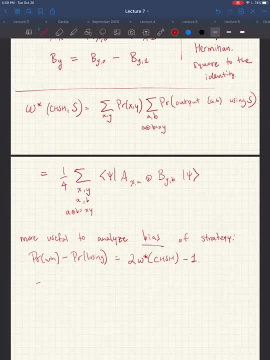 in this way, And the reason I'm going to use this is because I can write it in terms of the observables. So this is the same as one quarter divided by times the sum over the questions x, comma, y. I won't need to sum over the answers anymore. 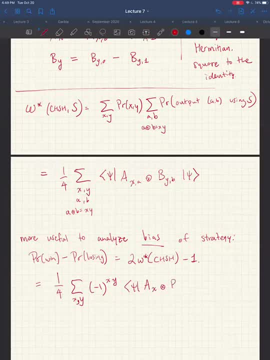 Because they've all been folded into the observables. So why you know these two are equal. this is you know. you can check this on your own Right. This is I mean. you just plug in the definition of observables and you'll see that both sides match. 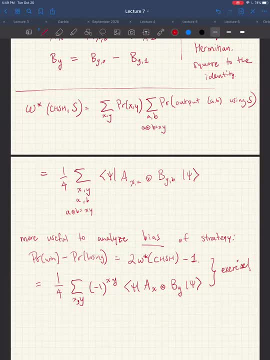 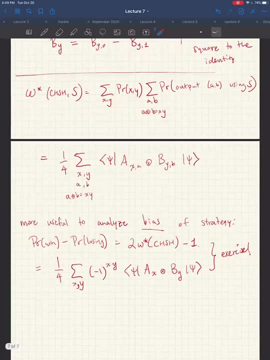 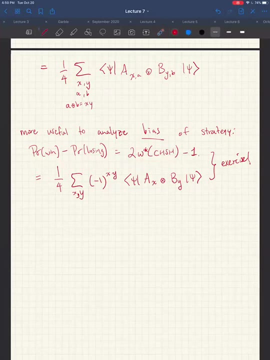 But you know, the point is that we have a slightly simpler expression to deal with, And if you know what the bias is, you can easily compute what the maximum winning probability is, for example, and go back and forth. So just one more question which is maybe kind of irrelevant. 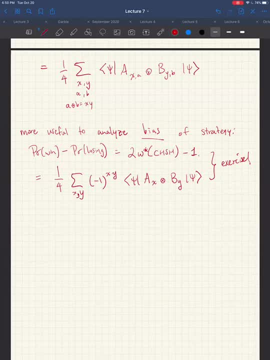 How do you know that they only make only one measurement? What if they measured the state 1,000 times? Yeah, Sure, So great question. So yeah, I mean, they can perform some enormous quantum computation, measure lots of things. 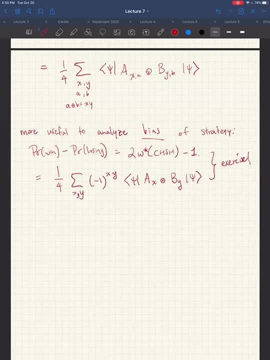 The point is, all of that can be wrapped into a single measurement Because at the end of the day, they're just giving you one bit And the probability of outputting that bit can be modeled as one And that bit can be modeled as a projective measurement on some state. 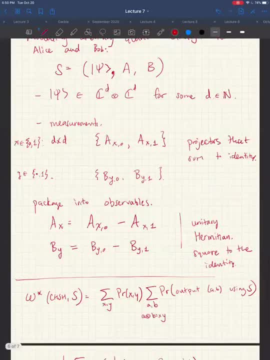 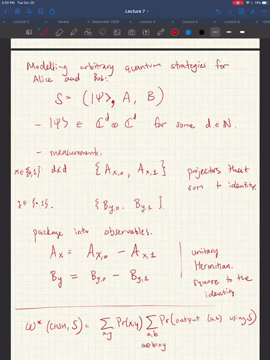 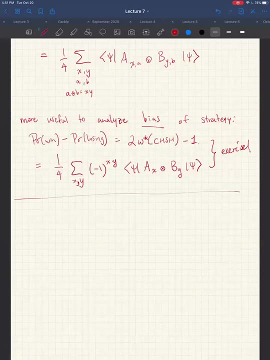 So, really, this way of modeling strategies, I mean, it encompasses anything they could possibly do within quantum mechanics. Okay, So, given this is how we, It walks up to you with some strategy. The first thing that we're going to prove is something called Searleson's bound. 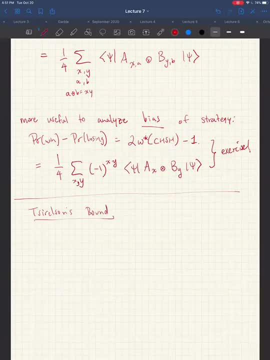 And this is really going to show that this 85% value is really the optimal value, That the quantum value of the CHSH game is at most cosine squared pi over 8.. Like there's no quantum mechanical strategy that can allow you to win with probability, 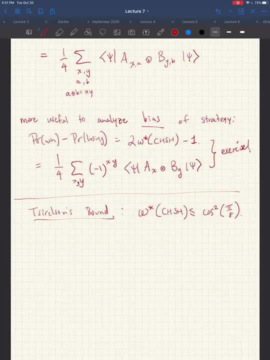 Let's say 1.. All right, So this number, this cosine squared, is actually equal to 1 half plus 1 over 2 root 2.. And this is equivalent to saying- and I'm going to write in terms of the observables: 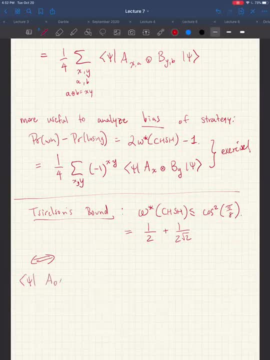 Is that This operator that's sandwiched by psi Is at most 2 root 2.. Okay, So this is the thing that you know. this expression, maybe you've seen it before if you've taken a quantum class before. 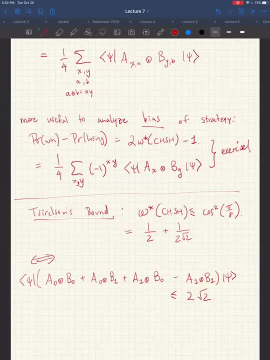 This is called Searleson's bound. It's, you know, named after this mathematical physicist, Boris Searleson, who actually, you know, just passed away pretty recently, like this January. But you know he's famous for proving a lot of things about these non-local games, like way before anyone else was thinking about them. 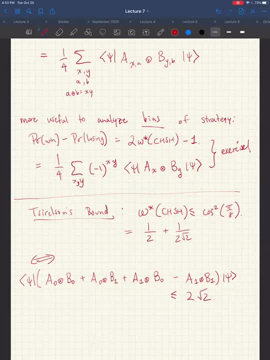 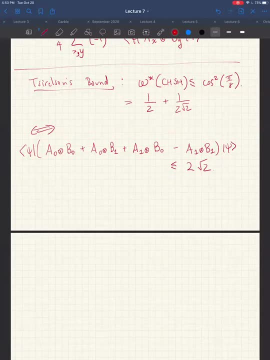 Okay, So. So, let's just keep on transforming. Let's just keep on transforming this expression into something that we can, you know, actually prove. So Are the minus and plus signs correct there? Yeah, there should be one minus sign in the when they both get question one. 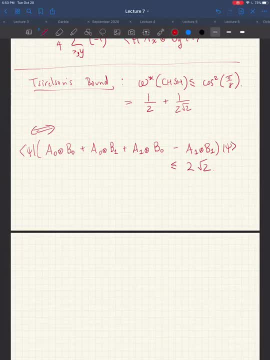 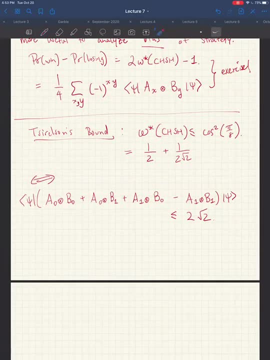 And then plus everywhere else. Okay, I'm not seeing that, but I'll look at it carefully afterwards. So Let's see So here. One way to see this is that You only pick up a minus sign when x and y, x times y, is equal to one. 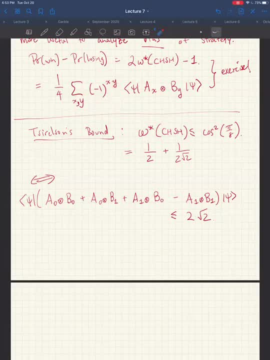 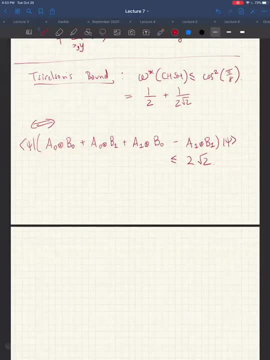 Fair enough, I forgot about that minus sign there. So so yeah, these, these two should be the same, And okay. So his bound is saying that this equation is, or this inequality, is always true, no matter what observables- A, X, B, Y- you choose, and no matter what state you choose. 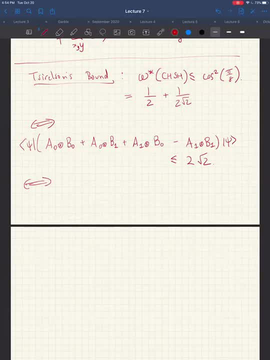 So This is equivalent, since you know you're also maximizing over the state. This is saying that the that the operator norm of this, you know of, of whatever matrix this is, is that most two root, two Right. 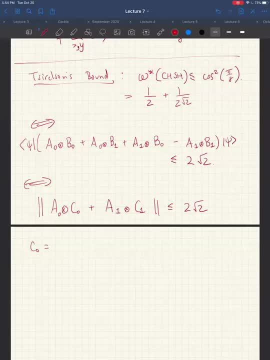 Okay, So if you plug in c 0 and c 1, what? what are these? Well, I, I've just collected the bees Right. You can verify that. if you plug in c 0 and c 1, as I've written them, then this is really just the original expression. 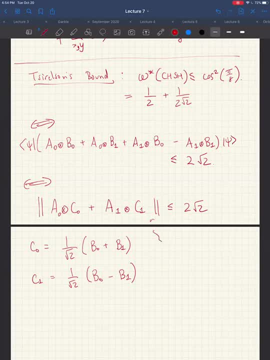 Right. So This is because the, This is because the operator norm of a matrix, this is just defined to be the Right, the you know you take the supremum where all possible states of you know M sandwiched by this matrix. 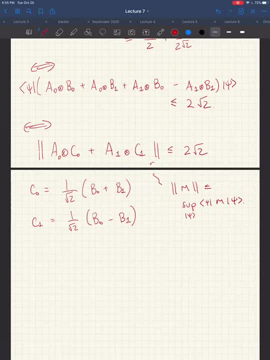 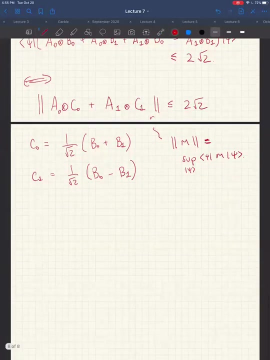 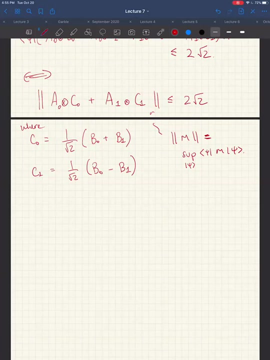 Like as long as M is a Hermitian matrix. but this is one definition of the operator norm. Okay, so this is really what we wanna prove. Just this statement, Henry. I think the bound on the right-hand side should be two Revit and two root, two. 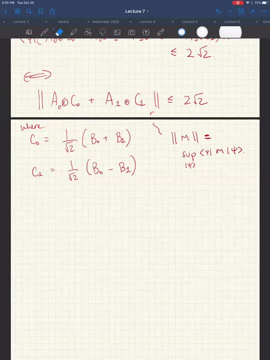 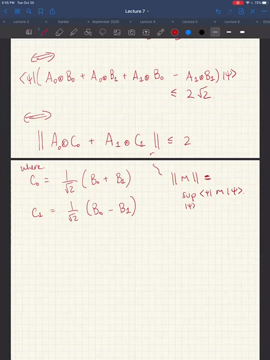 Oh, yeah, yeah, yeah, yeah, You're right, Because I've already divided by the root. two Good catch, thanks, Yep, Yep. so yeah, if you plug in C, hopefully, yeah, everything should match Okay. 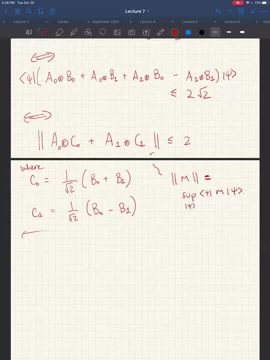 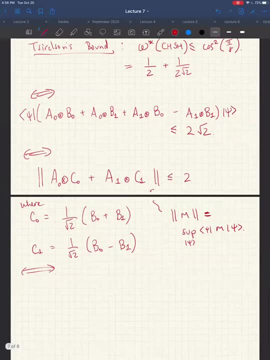 And I'm you know I'm gonna take another step right And you know, maybe this is like coming out of nowhere, but this is. you know really how he came up with it. How do you prove this? 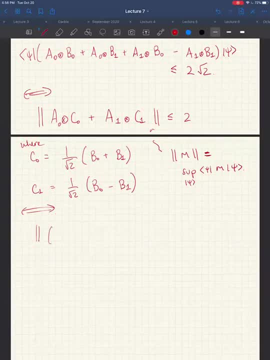 Well, I'm gonna prove another statement, which is that if I square this quantity, that the operator norm of the squared matrix is at most four. okay, You know why is that? Well, because, if you you know, this comes from. 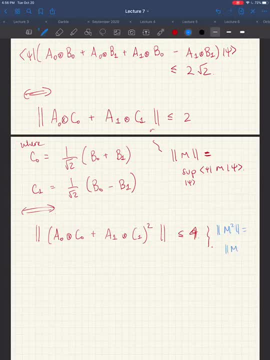 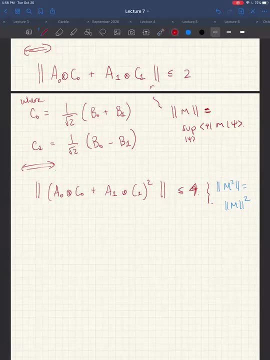 if you take the operator norm of a squared matrix, this is the same as the square of the operator norm. So if I prove that this, you know that this is less than four. then this must be less than two, right? Wait, why do we have two there? 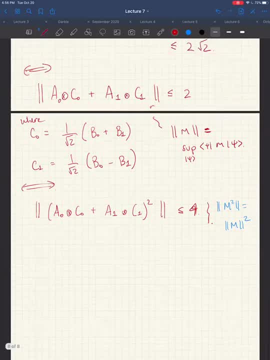 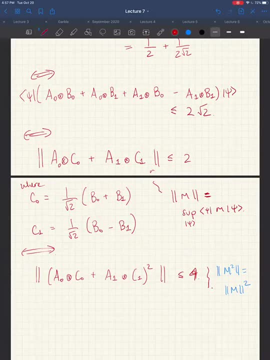 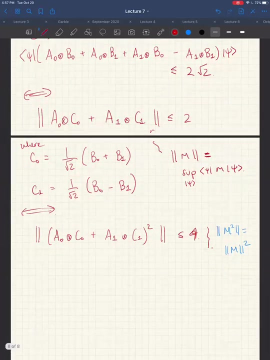 And before we had two square root of two. what is this? Oh, okay, So you, you divided by by in the Cs. Yeah, Yep, So the square root two moved into the Cs. Yeah, The reason why we're squaring this is because, actually, 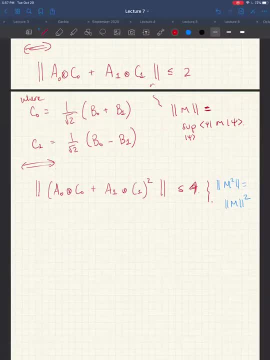 when we expand it out, we're going to get some nice cancellations. So so let's start opening things up. We're going to get a zero squared tensors C zero squared. A one squared tensor C- one squared. And then we're going to get a bunch of cross terms. 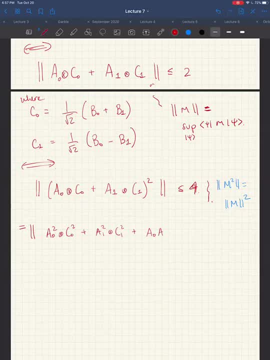 So we'll have a zero, a one, tensor C, zero, C one plus a one, a zero, tensor C, one, C zero. And you know, just maybe obvious, but these things are not the same, because A zero and A one. 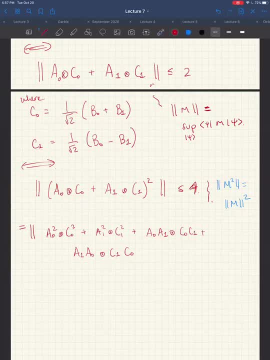 C, zero C. one don't necessarily commute right, So we got to keep track of both of them. So that's, if we open it up, that's what we get. And now we're going to start taking advantage of the fact. 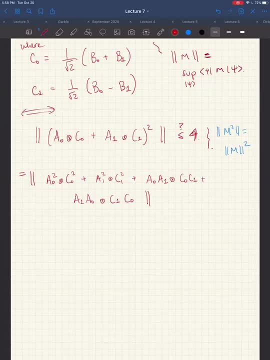 that we know the A's and B's are observables that square to identity. So let's, let's evaluate each term separately. So A zero squared tensor, C zero squared, this is identity. So A zero squared tensor, and we just have to square the C zero thing, right? 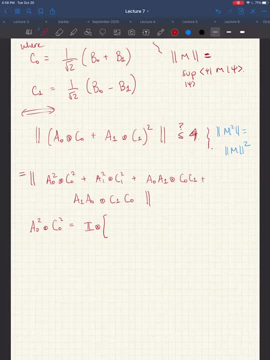 So this is this is going to be: you're going to pick up a one half on the outside right, That's you square the one over square root two. We're going to be zero squared plus B one squared, And then you're going to get the cross terms right. 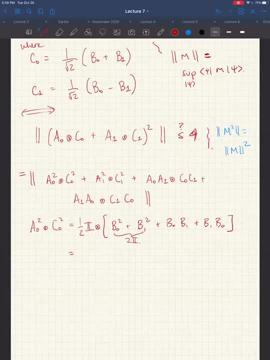 Uh, we know that this is also two times identity, So we inclined that we get identity plus one half P zero, p b one plus b one v zero. All right, Next square term: Using be zero be one: uh equals zero. be zero be one. 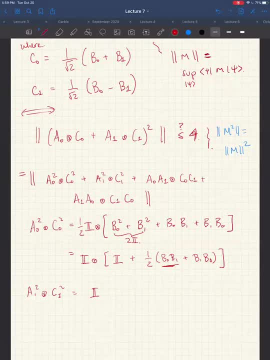 This one here, Yeah, and the same for the other one, Cause if it was a Z basis, it would be. you would have a zero one, like a product between zero and one right. Oh, so these are the observables corresponding. 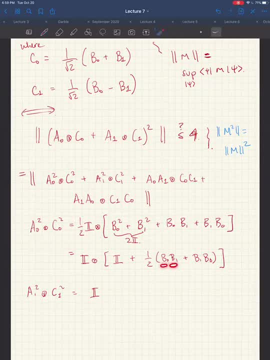 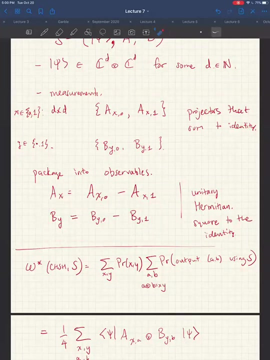 to the two different questions. So B zero, B one are observables. So we don't know what the relationship between the two are, And so let me go back to our definition. We just know this, Right, Okay, yeah, and if it were, a BY zero, BY one? 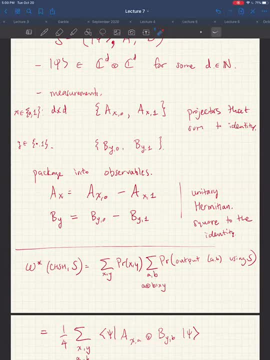 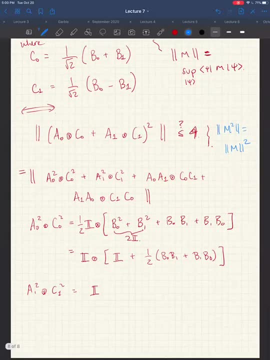 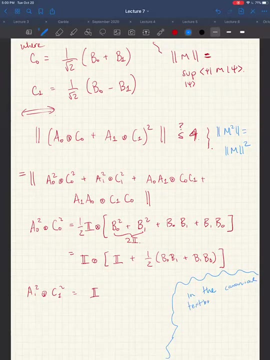 this would be zero. Yeah, Okay, yeah, I'm confusing it, Okay, sorry, Actually, yeah, actually it might help, like as a mental model, just in like the canonical textbook strategy, You know actually, yeah, you might find this helpful. 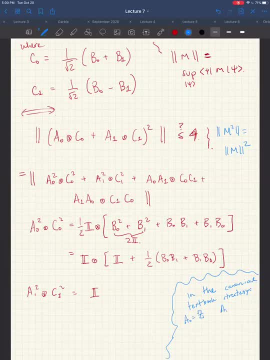 So A zero should be Z, A one should be X, like the poly operators, And then B zero is equal to this, like you know, one over square two. you know Z plus X, And then the B one is equal to Z minus X. 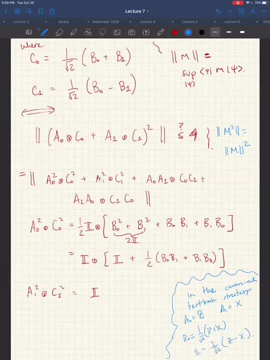 So if you wanna, like sort of do a sanity check on what this should be, then you can plug in these operators And see what you get. But in this arbitrary strategy, we don't know what it is. They're just like you know. 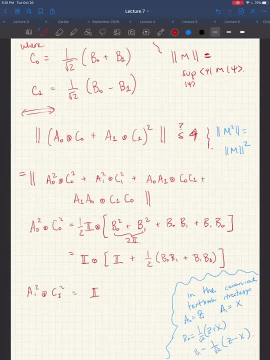 arbitrary D dimensional observables, but we do know that they square to the identity. Okay, so you know. just working out the algebra, you get nearly the same thing, except you pick up a minus sign, Right, Okay? So if you sum these up, 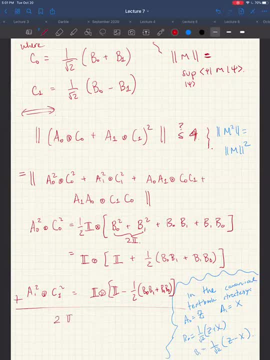 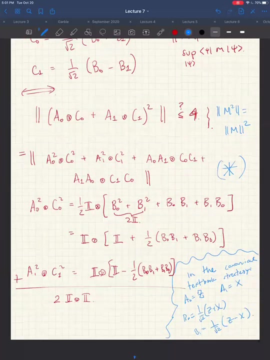 you get two times the identity. I believe Right. Okay, so I'm going to give. I'm gonna call this equation star, so I'll refer to it. So star is now equal to: we have two times the identity, Right. 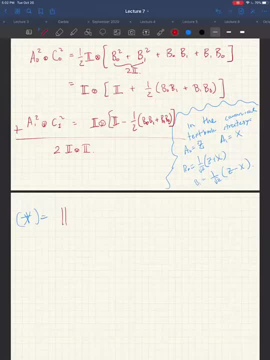 Tenser identity Plus, you know, still, we still have these cross terms, Oops. And now I'm gonna use the triangle- inequality for the transfer, the missالم, because you know, it's just a beautiful thing to write. 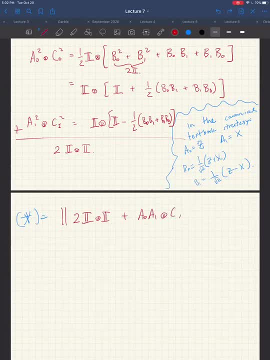 but it's almost you know the, just the upper half of a line and you're just sort of you know, you're like it's like you're gonna write this these terms, And then the other side, you're gonna write this these terms. 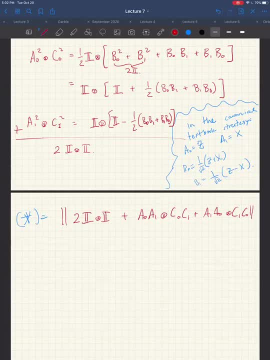 Right. And then the other side, you're gonna write this, this, this angle, you're gonna write this, this, this. So you're gonna write this, this, this, this, this, this, this for the operator norm, So we'll have you know, two times the identity. 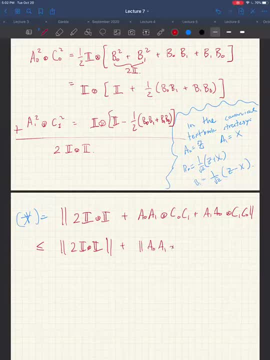 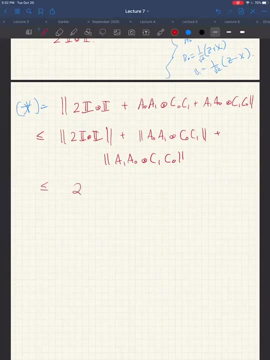 plus a0,, a1, right. And we know that the operator norm of twice the identity is at most two right. Well, it's equal to two. And also we know that the operator norm of a tensor product is just the product of the operator norms. 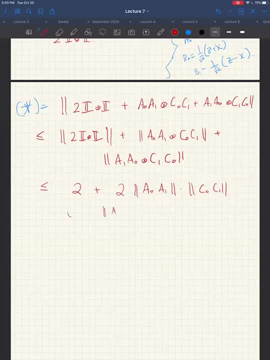 And I've used just a couple of facts, like you know. for example, like if you have the product, it doesn't matter which order you compute them in, For example. Okay, So we're almost done, We just need to start bounding these operator norms. 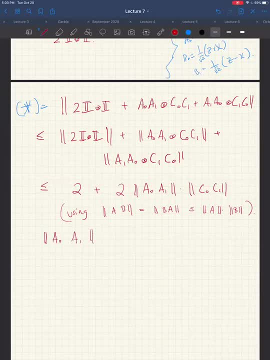 So one thing we know is that a0 times a1, what's the operator norm of this? Again goes down theII matrix. I would say at most one, because it needs to work. All right, that's a good student answer. 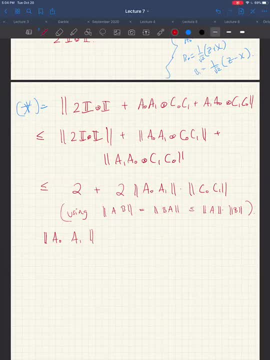 So we know a0, a1 are unitaries right And unitaries have, So the operator norm has to be exactly one. All right and good. So now we just need to compute C zero times C one right. And here we just have to expand out what this is. 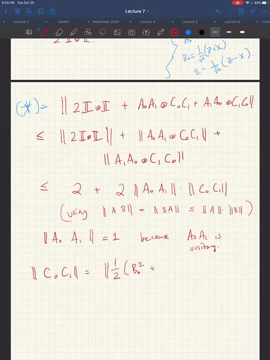 So this is B zero squared plus minus B one squared plus these cross terms. Right, so we know that these are both identities, so they cancel out to be zero. So this is equal to one half B one, B zero minus B zero B one, or maybe the other way around. 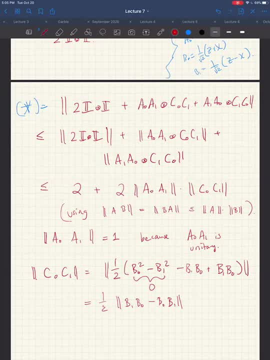 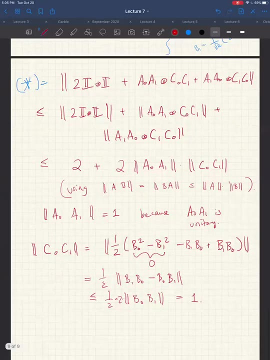 but it doesn't really matter And the you know, here we don't. again we're gonna use the triangle inequality. So we get pick up a factor of two and but this is all equal to one. So, just plugging everything in, we get one here. 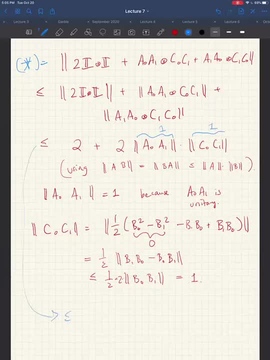 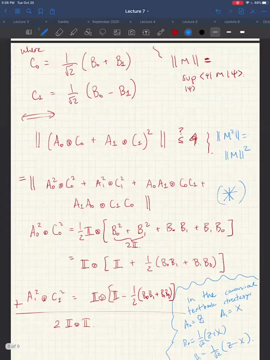 we get one here and we finally get, we get the desired bound, which is: all of this is less than four, and it all works out as we hoped. So we, we've deduced that, you know, we've deduced the, the Searleson bound, okay. 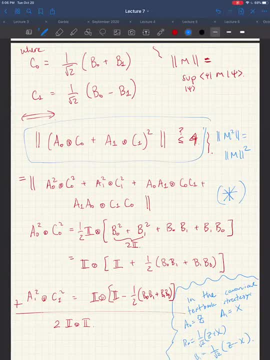 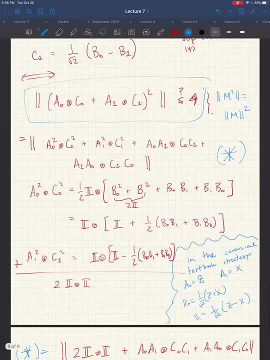 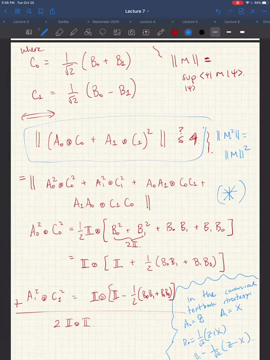 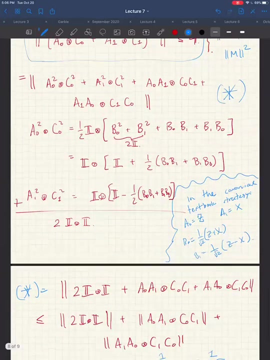 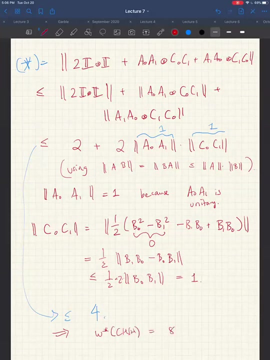 And this shows in kind of, you know, just by plugging through this algebra, that you know 85% is point 4% is the best you can do in this CHSH game, Okay, so maybe let's take like a, you know? 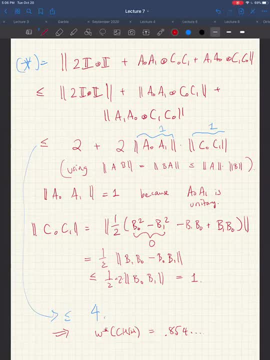 for these course materials. you know five minute break, so let's come back at 5- 11 and we'll continue on. you, you, you, you, Thank you. You made me explain that triangle inequality step one more time. It doesn't minus sign. You make it weird. 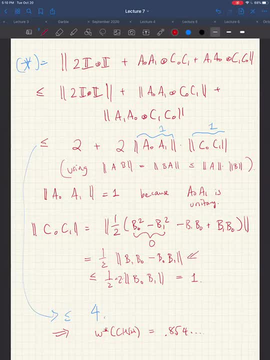 Let's see You mean this one here. Yeah, I guess you can just treat it as like you know. this is like B1, B0 plus minus B0, B1.. Yeah, And just treat the minus B0, B1 as like just another operator. 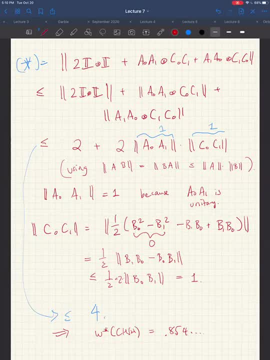 And I guess the other thing is that the operator normally doesn't have a number. It doesn't have a number. The norm of minus an operator is just the same as the operator norm of the operator itself. So like norm of minus M is equal just to the norm of M. 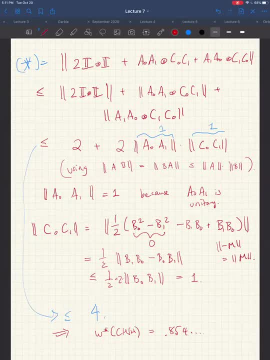 Yeah, So does that make sense? And also, you know, A plus B is at most norm of A plus norm of B. So if you put those two things together then you get the triangle inequality statement. Thanks, Yeah, Okay. 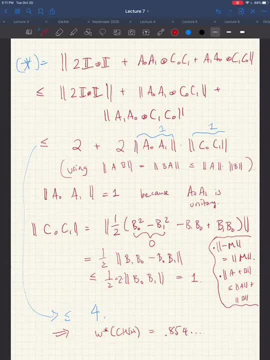 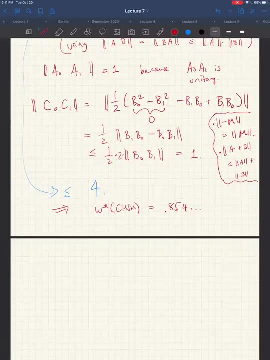 Yeah, Any other questions about, like the this derivation? Okay, So let's move on. So we've seen like there is a non-trivial upper bound on how well you can do, And we're actually going to kind of build off of this proof. 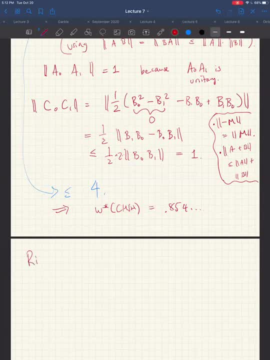 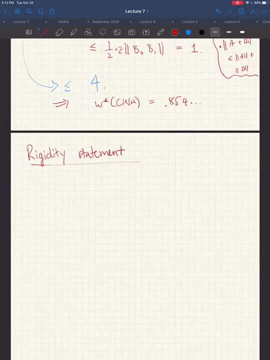 to prove this rigidity statement. Okay, So, so, just to keep things simple, I'm going to like, analyze, show, like rigidity for the case of when you have a strategy that exactly achieves the optimal value. So let's say that someone walks up to you. 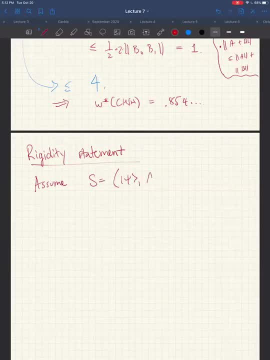 with an arbitrary strategy for the CHSH game where the value is, let's say, let's say, equal to, you know, cosine five or eight, Then we want to do something about the. you know the structure of the strategy. 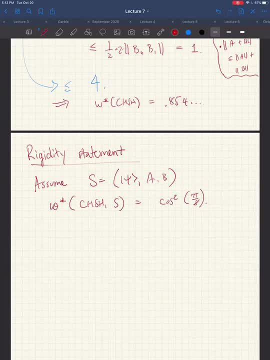 Like I'm claiming that it's essentially the same as this canonical qubit strategy. but then you say: well, how can that be possible? Because this strategy S could be D dimensional right, Like it could, or D equals to a gazillion. 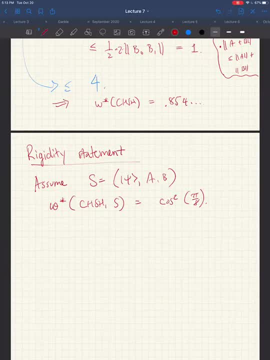 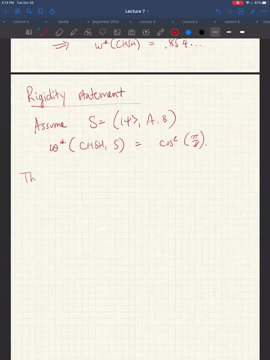 right, Which is much greater than D, equals to two. So I have to explain what exactly I mean by them being the same. So this is the exact CHSH rigidity And the same is a little technical, but we'll like kind of unpack it and see why it makes sense. 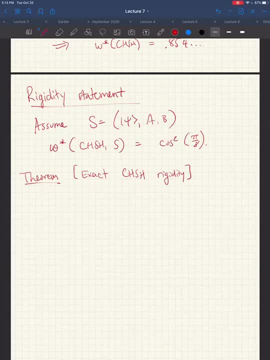 So so you know, suppose that you have the strategy like this, then there exists. Okay, So actually, before that, let me, let me just draw a picture. So you have a state side and let's imagine that it's on. 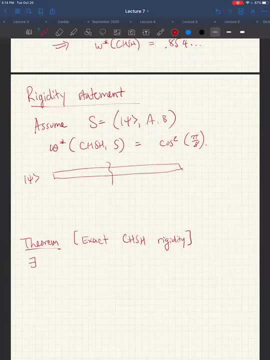 it's on two ridges, You know. each of them is a D dimensional, Each side is a D dimensions. right For Alice and Bob. And I'm going to. I'm going to give Alice's space a name, I'm going to call it script day and I'm going to call 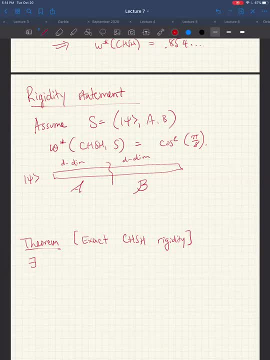 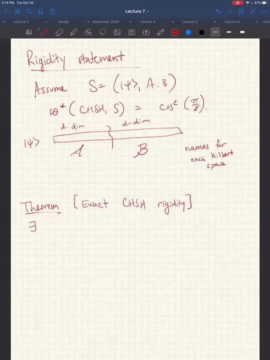 Bob space, script B. So these are their register names, Right, I'm going to try my best to like write the scripts in the correct curly font, And and so the. so we view, like the, the observables a, zero, a one as acting on Hilbert space. 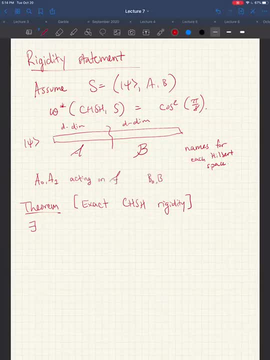 script a, and then B, zero, B, one as acting on space script B, And I'm going to use these, these register names, to just keep track of when different operators are acting on which sides. Okay, So back to the theorem. it says that they're going. 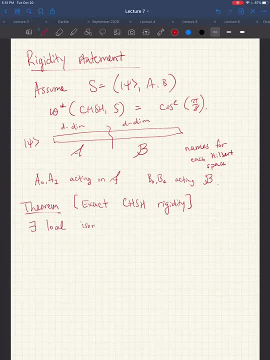 going to exist local basis changes. So, technically speaking, there's going to be an isometry. I'll I'll explain what that one isometry is later. It's you know. you can think of an isometry as a unitary. for now, 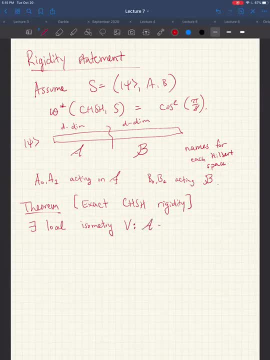 So it's going to be some change of basis that maps, say, Alice's space into a new space And I'm going to call script a one and script a two. There's going to be another isometry, but this time for Bob. 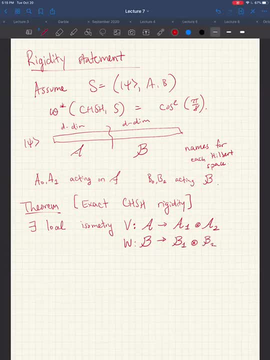 and it's going to map into B one and and B two. Okay, What are these? a one, a two, B two, B one, B two. Well, the a one and B one are going to be isomorphic to C two. So this is where the qubit is going to appear. 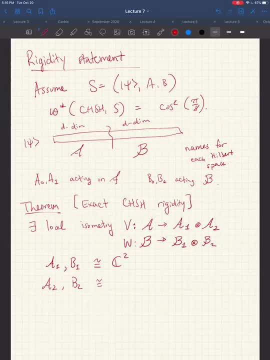 And then the a two, B two is going to be isomorphic to some other space CD D prime for some D prime that I don't really care about, It's just some integer. So It's like a little local basis change where you kind of 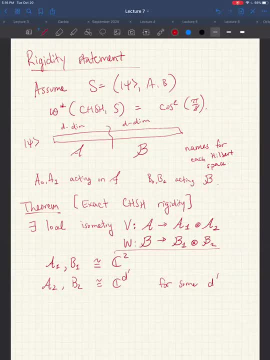 like re, you know kind of reorganize the basis States where you've kind of identified. So you know, when you apply V tensor, W two to these two spaces, you're you're going to see a slightly more complicated space where there's 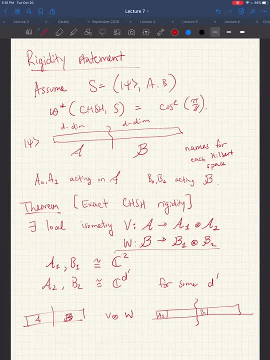 a one and B one and B one here, And this is going to be a two dimensional space. It's like enough to hold one qubit and there's going to be a two and B two, and this is going to be a larger space. 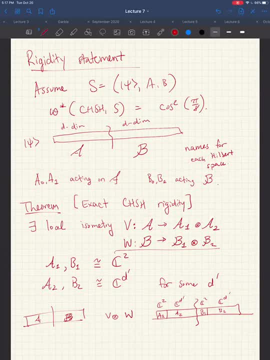 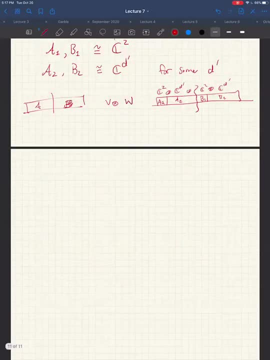 but we call it the junk space because we don't really care what's happening here. Right And and put together, all of this is going to like this: this space is going to be, you know, C two tensor, CD prime tensor. 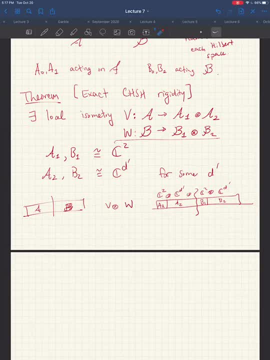 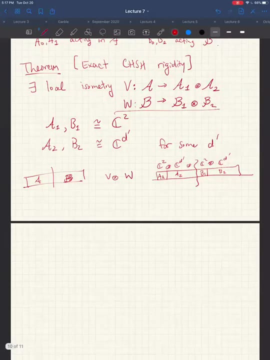 C, two tensor, CD, prime. All right, So that's what these linear maps are going to do. Okay, So? so what do we do with those linear maps? Well, it's basically kind of like you can think of it as changing the basis, so that when 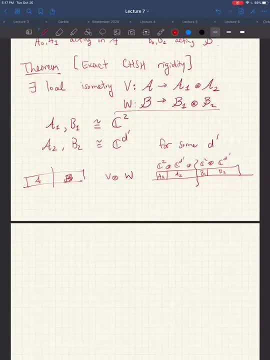 you apply it to the strategy, you actually see that the strategy was just really hiding the, the original canonical qubit strategy. So if you define a new state which is like I'm going to take this V, tensor W and apply it to, 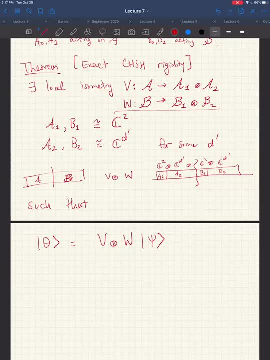 the state that's used by Alison Bob in this strategy, then the state such that if you let you know theta equals this rotated state. then you see that it's actually factors as an EPR pair between registers a one- and B one tensor. 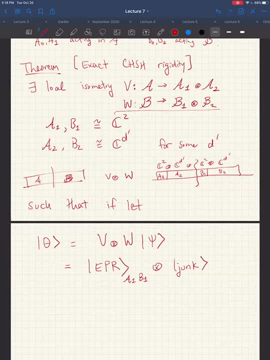 some junk state, right, Junk is, we don't actually care about characterizing, It's just some other state that lives in registers a, two, B, two, Right, So we've. so this, we've you know, from this arbitrary state. 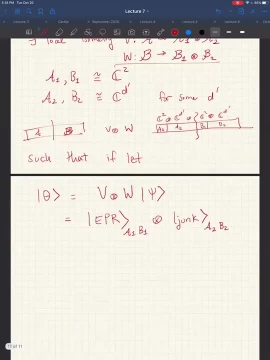 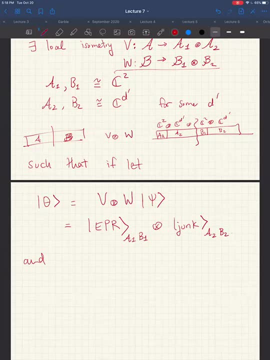 Psi, we've picked out the existence of an EPR pair. How can you guarantee that it's pure in that way? Well, it, this, this theta is going to be pure because Psi is pure. We're assuming size pure and you're applying an isometry or unitary. 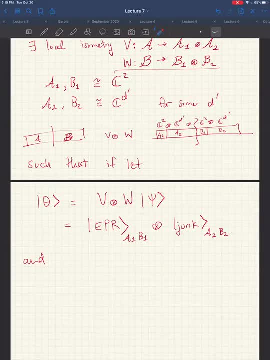 So that will keep the purity, So, um, so, therefore it has to be pure And in fact it's going to factor in this way. So that's maybe the surprising thing. I mean to pick up on that, like maybe there. 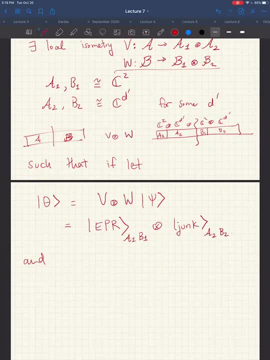 how do we know there aren't really complicated correlations here that prevent you from doing that? Oh, you mean there. how do you know There there might not be entanglement between these registers and this register. Uh, sure, Yeah. 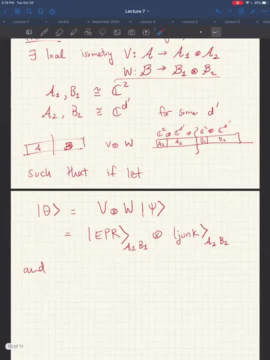 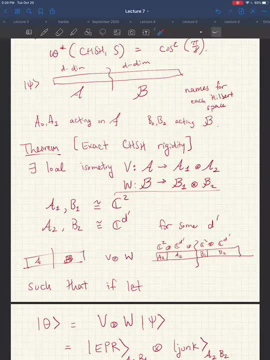 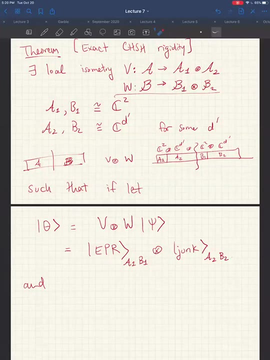 Oh well, it's because you're starting with the constraints that they're winning the CHSH game, perfectly, So it's so. this constraint is so strong you know that there cannot be any like. there must be somewhere in this crazy D dimensional space that they're starting out with. 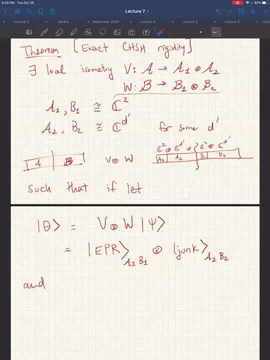 You can identify an EPR pair and extract it out, And you know all the action is going on on this EPR pair. So are you assuming that or you're proving it? We're proving it, So, um, okay. 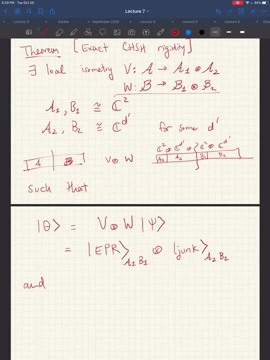 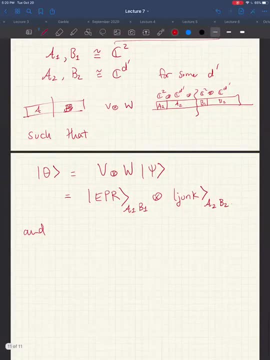 Well, like so. so this is the conclusion. sorry, sorry, go ahead. Um like, am I correct in? status is stating that once we prove that we have an EPR uh state there and by the monogamy of 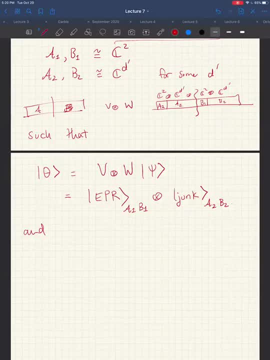 uh, entanglement. we can now state that these two qubits cannot be entangled with anything in the junk state. Um yeah, Although you don't even need to go that far, Like the fact that I've written as an EPR pair that are like sort of just by definition. 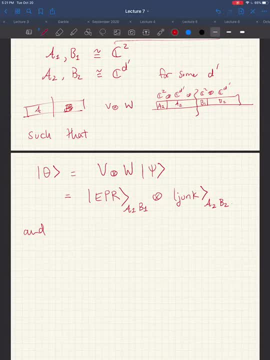 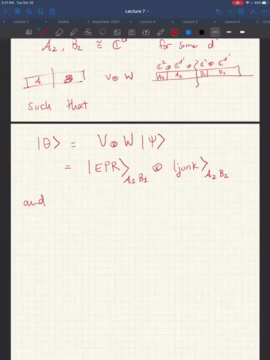 it cannot be entangled with anything else. Okay, Um. so there's one more part to this theorem, which is to say: well, what about the operators Um, so, the, this will look like this: So it, um. 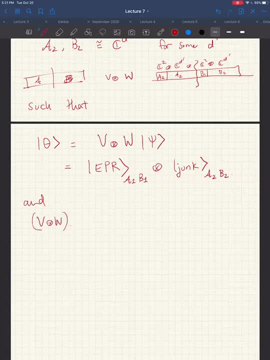 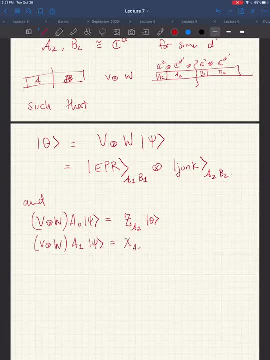 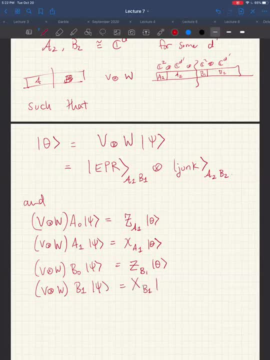 but let's, let's parse what it means. Okay, So let's, let's just start with this. It's saying: you know, consider two different ways of doing something. Um, Imagine that you took the state psi that Alice and Bob started with. 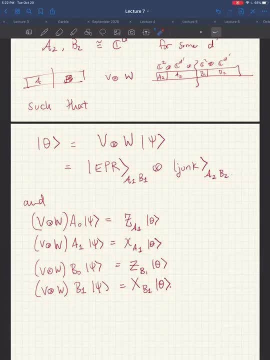 and Alice just applies as a unitary this operator a0. So remember a0, it's an observable, it's a unitary, so you can just apply it to the state. A0 only acts on Alice's part of psi, right. 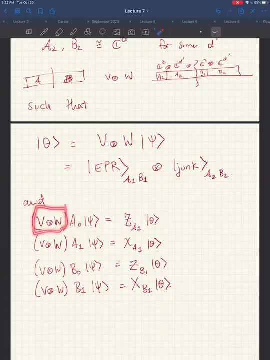 So you do that and then you apply this basis change. This is the same thing as if you started with the basis change state, like you change the state first and then, on the EPR pair, you apply the Z operator on the qubit. 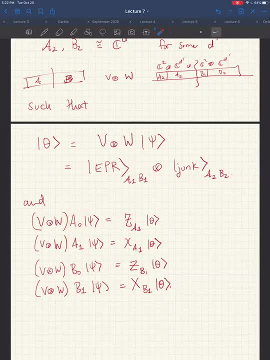 So it says that really as complicated as a0 might look after you've done the basis change, all it's really done is just performed a one qubit operation on the EPR pair and it didn't do anything to the junk state. 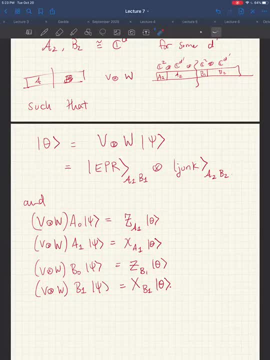 And okay, so the rest of this should make more sense. So then you say: well, what if I did a1 instead of a0?? Under the same basis change. it looks like an X operator on the EPR pair on Alice's side. 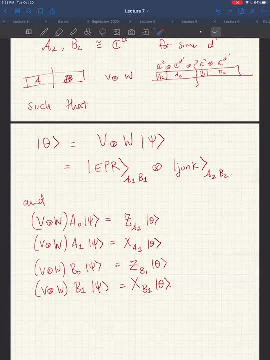 And then same thing for Bob's operators. Like there is a basis change that looks like a Z on B1 on this part or X on B1.. Z and X and not the Z plus X and Z minus X. Good question, So you're right. 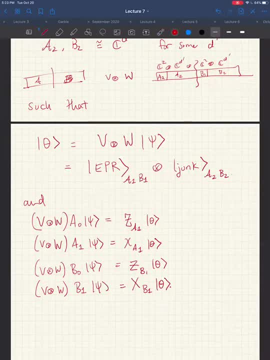 So you're saying, well, this doesn't exactly look like the canonical strategy, but it turns out that, so I'll write it in blue. There's like another, because there's a local basis change where so there's a two by two unitary U. 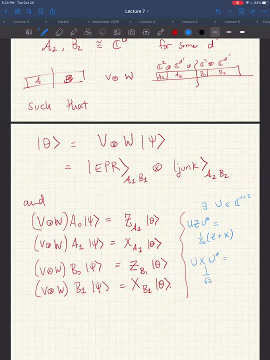 where you can really map X and Z to Z plus X and Z minus X. So I'm just kind of folding it. I'm already folding it into these local isometries. So actually I'm not sure if you can see it. 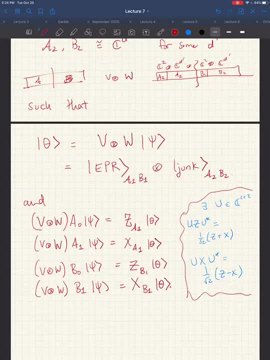 I'm not sure if you can see it. I'm not sure if you can see it, Okay, So in this way it actually makes the description of the CHSH strategy a little more simpler, because you just say: oh well, Alice and Bob. 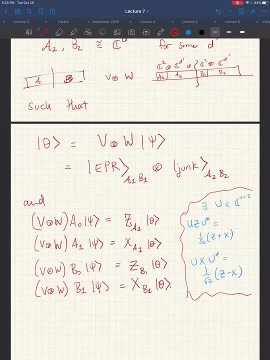 are just using Z and X, Z and X, but Bob will have to first perform a basis change to do that. So did someone else have a question? Okay, So that's the statement. I mean it's kind of long, but hopefully it should. 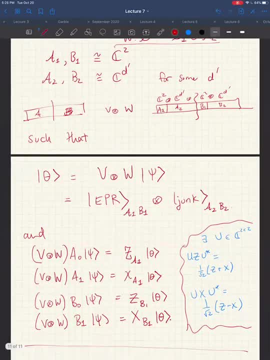 intuitively. it just means that we've really identified in this arbitrary strategy that succeeds optimally in CHSH, this qubit, this EPR, this ANT and this CASH state and the single qubit unitaries that act on the EPR state. 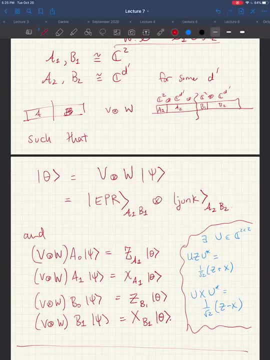 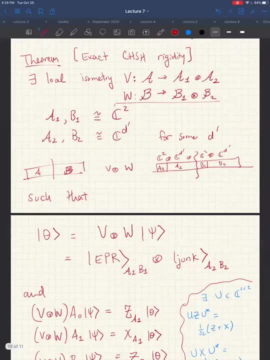 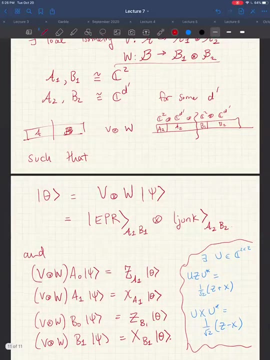 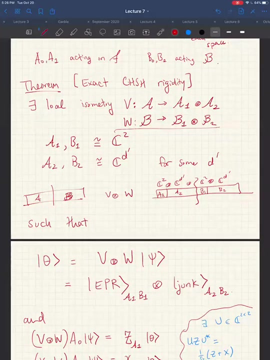 And you know, there might be this other junk state, but nothing interesting is happening there. So can we say something about the uniqueness of these to be in W, The uniqueness of the V and W? Oh, I guess it's. Or the finding for conditions? 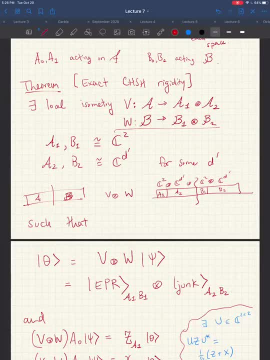 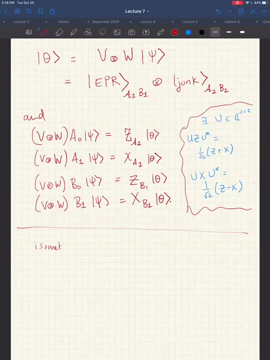 to then apply something about the uniqueness. Let's see, They're not unique for some trivial reasons, Like, for example: so they're isometries, Oh, okay, Oh, at first I should say what isometry is. So isometry, it's just a length preserving map. 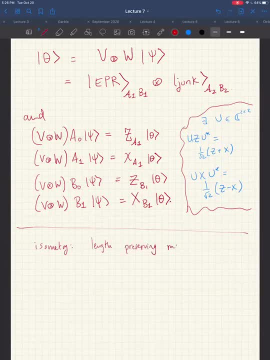 So let's say you have an isometry from space A to space B. It just means that the dimension of B has to be at least the dimension of A, And then for all X in A, the norm of V applied to- Sorry, the norm of X has to be the same. 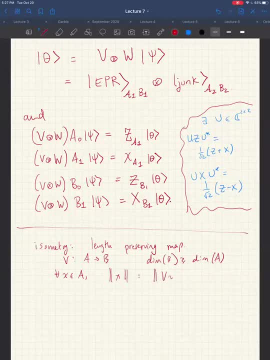 as the norm of V applied to X. Right, You know one way of thinking about what an isometry does. it's sort of it applies it. like you know, you can take the state, the input state. you tack on some ancilla zeros. 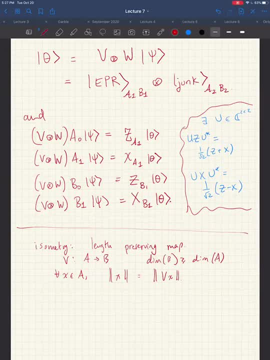 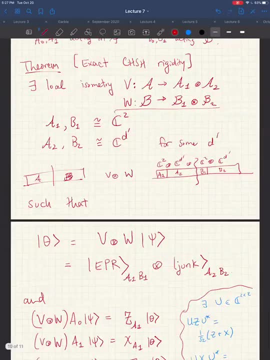 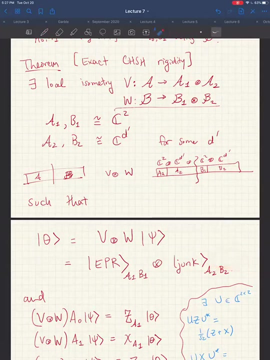 and then you apply a unitary on that bigger like concatenated state. That's what an isometry is. So one thing that this, these isometries, could always do is just tack on additional zeros On to the junk state, And so it wouldn't be unique for that trivial reason. 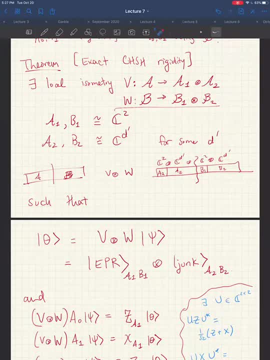 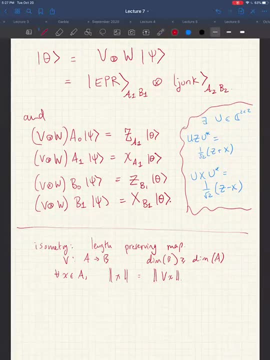 Right, right, okay, So, yeah, so you know, I guess it's. you know it's a big, it's sort of a lengthy theorem, but it's worth sort of like mulling over and sort of trying to see like. 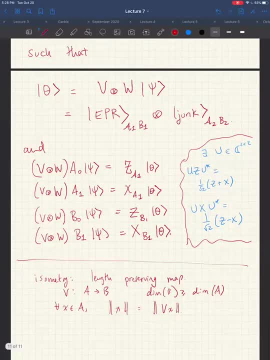 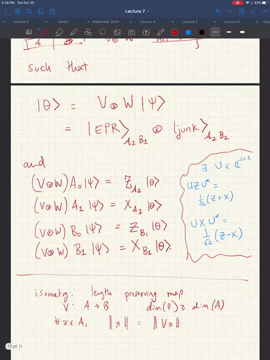 I mean, it's really constraining it, Like it says that you can really extract out this, the simple strategy, no matter what crazy strategy you might've walked up with, And so so how do you prove such a thing Like, how do you locate this EPR pair to begin with? 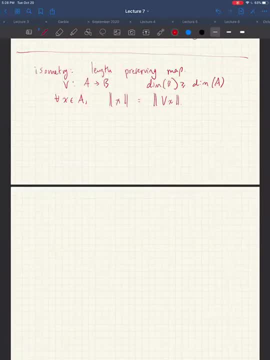 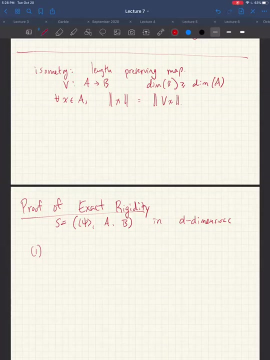 And so the proof of this theorem goes in three steps. So you know, again, someone hands you this arbitrary Psi A, B and D dimensions. The first thing we want to establish, and the most important thing, is that you want to. 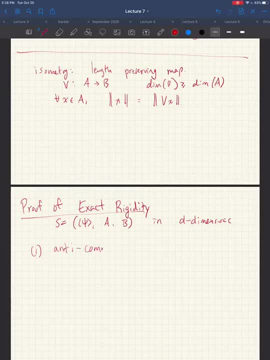 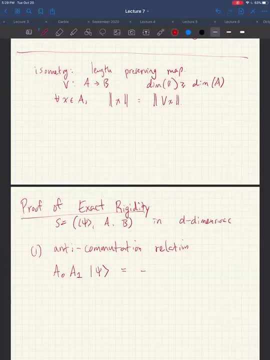 And it will turn out that if the strategy actually wins the CHSH game perfectly, then in fact it forces these observables to have this anti-commutation relation. Like A zero times A one is equal to minus A one. A zero as long as you're operating on the state. 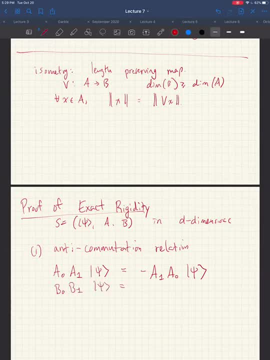 And similarly for- and you know, as a sanity check, this should make sense for our actual operator, like for the canonical strategy, because if A zero is Zed, A one is X, then we know that they do in fact work. 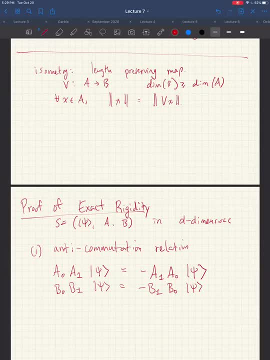 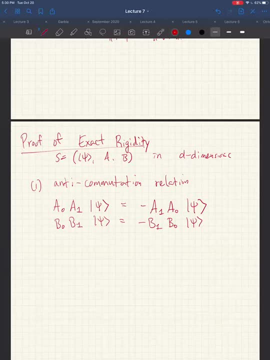 They do, in fact, anti-commute. So so this is like a legitimate thing to prove. And another thing is it's kind of like it's kind of weird that you would be able to deduce this right Like in the actual game, you know. 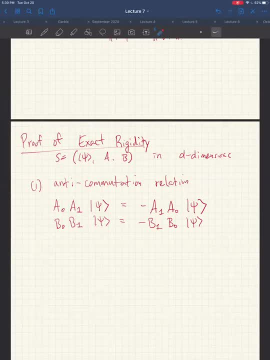 when you're playing this game with Alice and Bob, you know they're only ever applying one measurement at a time. They're either doing A zero or A one. They're never doing A zero and A one at the same time. yet Somehow we're able to deduce some relationship. 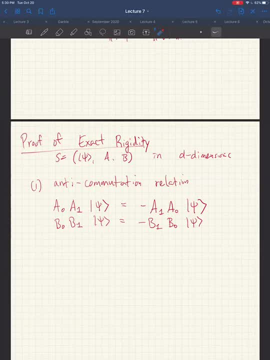 between those two operators And really that's at the crux of it. So let's say, you, you, you establish that. Then, from from this, this is already enough to to help you identify a qubit within, within their strategy. so 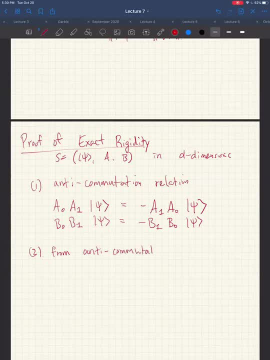 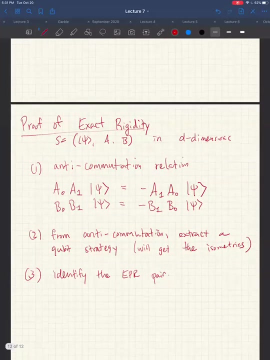 So we'll get the these isometries V and W, And then the very last step is is just to identify the EPS. So the first step is to identify the NPR pair. Okay, So, So, let's, let's carry out these steps. 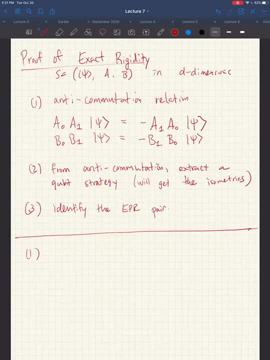 Let's, let's, let's show that anti-commutation muscle. Okay, So let's start with the fact that this strategy is optimal. So then it actually means that this previous expression saturates zero sense bound. So you know, not only is it, at most two. 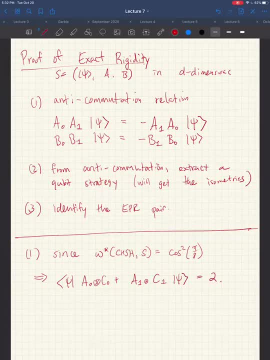 it's actually exactly equal to two. Okay, and we're gonna just get a lot of mileage out of the fact that this is exactly equals. So let's see. what do I want to argue here? The first thing I want is: I want to argue. 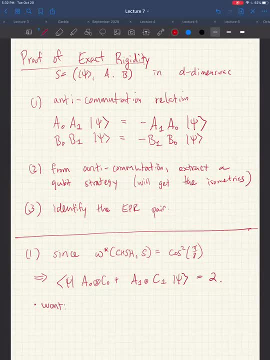 okay, so C zero. remember that C zero is equal to zero. C zero and C one are like these linear combinations of the B zero, B ones. You don't know immediately that C zero and C one are observables or even unitaries, right. 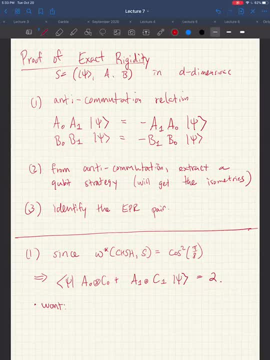 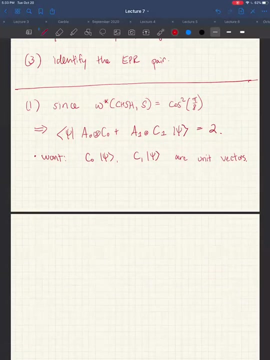 So we actually first want to establish that they are in fact unitary. So we want to know that C one times the state, C zero and C one times the state are unit vectors Which we don't immediately know off the bat. So let's see. 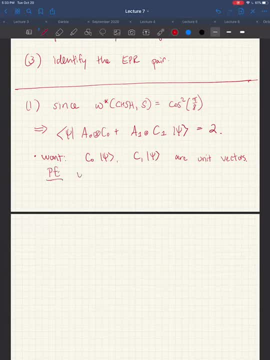 Okay, so to prove this, we're gonna use the Cauchy-Schwartz inequality. All right, so what's Cauchy-Schwartz Like if you have two vectors? they're just a reminder, like the inner product. 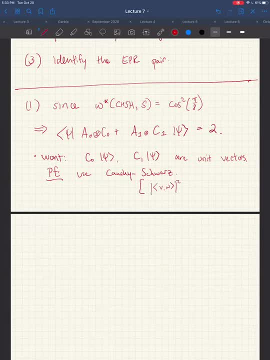 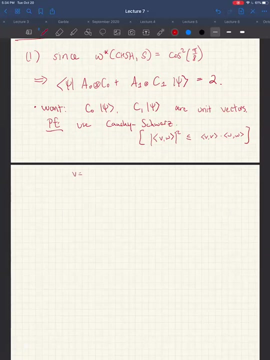 between two vectors of V and W. if you square them, it's at most the inner product of V with itself times the inner product of W with itself. So let's use, let's say, that V is equal to the observable A, zero times Psi, and let's say W is C, zero times Psi. 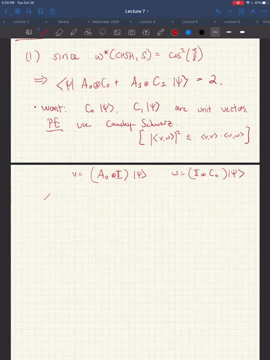 All right. and if we apply the Cauchy-Schwartz inequality, then this: A zero tensor C zero is at most. So this is Cauchy-Schwartz, It's the inner product itself. So that'll be A zero squared tensor identity times. 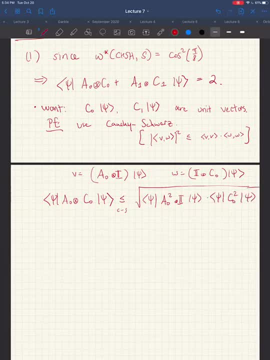 C zero squared. I'm gonna leave off the identity. This is equal to one right, Because A zero squared is the identity, And now we just have to figure out what C zero squared is. but we actually calculated it before, So I'll just find it out. 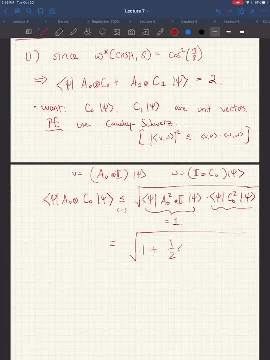 Like you know, if you work out the algebra just by plugging it in, it's these cross terms All right. and if we do the same thing for the A one and C one term, this is at most everything's the same. 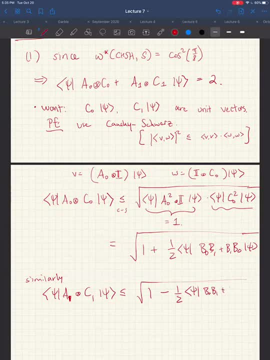 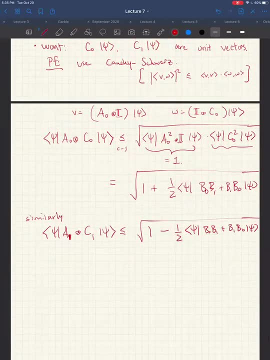 except we have a minus sign. Okay, and now let's use the fact that they saturate the Serosin bound, right? So if I call those quantities one and two, I have that one plus two is equal to two, right. 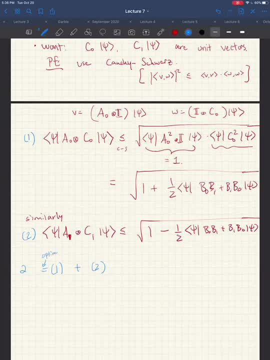 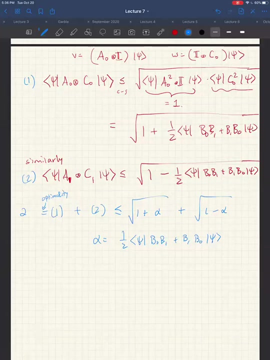 This is from optimality, right, But there are also at most this: one plus alpha plus one minus alpha. Alpha is just this: one half B zero B. one B, one B zero, Right, but the only way that I mean you can just like you know. 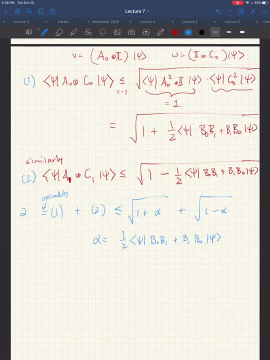 deduce this or run it through Mathematica or whatever. This is only possible if alpha is equal to zero. Okay, and it's not hard to see, but you know you can take my word for it. So if alpha is equal to zero, 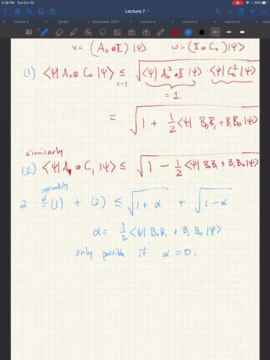 I mean already that should be really suggestive, right, Like it should tell you that this thing is- I mean, this is looks like the anti-commutator of B, zero, B, one, right? So we're almost there, but what it tells you is that 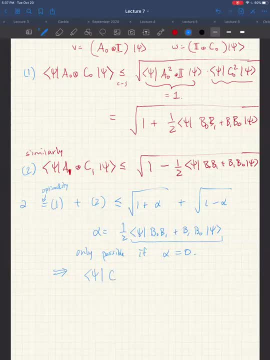 what it tells you is that C zero squared and C one squared is equal to one, Or in other words, that these vectors have unit norm Right and like that was the first thing that I wanted to show. So C zero and C one. 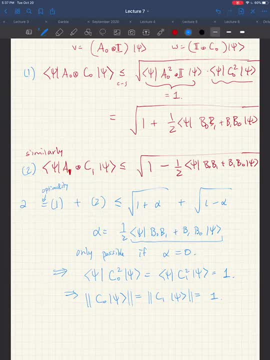 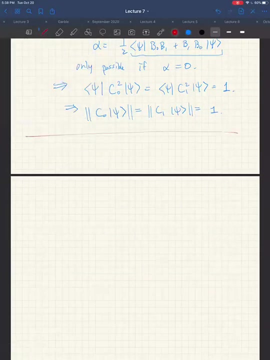 like they look like unitaries, Right, Okay, Okay. so we're basically there. We just need like a couple more things. So we know that they have unit norm. So now let's look again at this, at this, this equation, right? 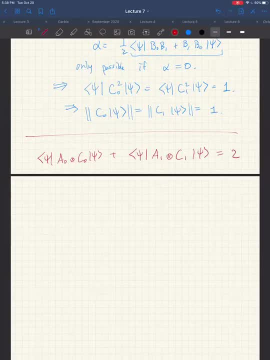 The fact that we have saturation of the serial sin bound. This is, you know, these two sum to. they're equal to two, But this is the inner product between two unit vectors. right Like A zero, psi has norm one. 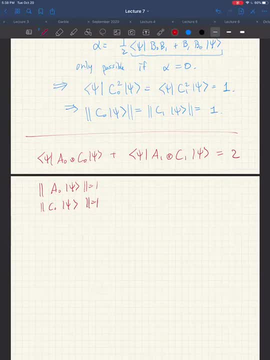 C, zero psi has norm one, as we just proved. So when you take the inner product of two unit vectors, their norm can be at most one right, And you know the same thing here. So this tells us that A zero tensor. 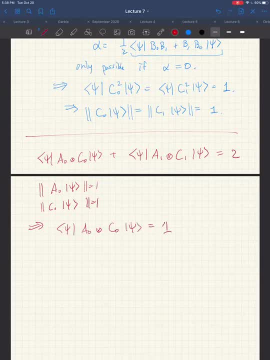 C, zero psi, like they both have to be one, Like they can't be anything else And they couldn't be any other than a number. But then, but what does that tell us? I mean, you can view this as the inner product of 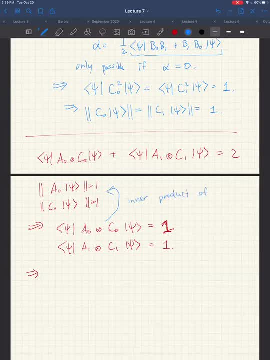 inner product of these two vectors. And you know if, if you take two vectors, unit vectors, and you take their inner product and they have inner product one, that must mean they're the same vector, Like they have to be exactly the same. 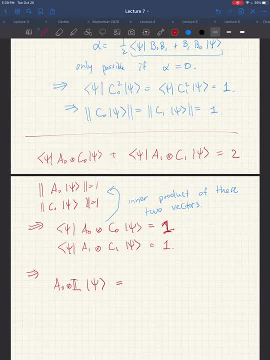 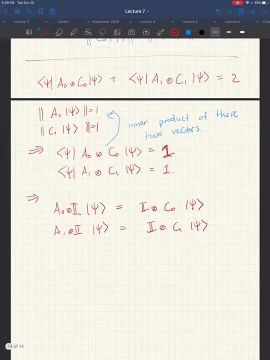 So we get this really cool fact that A zero times psi is equal to C zero times psi And similarly, and the reason this is cool is this: this is called operator switching right, Meaning that here's an entangled state. If you apply Alice's observable, A zero as a unitary. 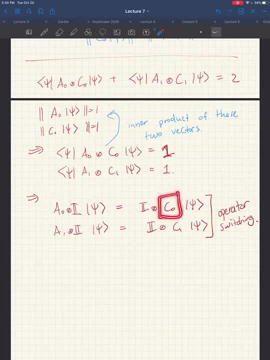 that results in the exact same thing as if Bob applied C zero On his side of the state, or you know, or whenever you see an A one, you can switch it with C one, or vice versa, And that's really useful. 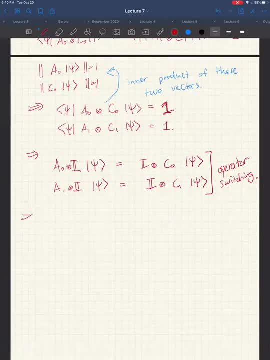 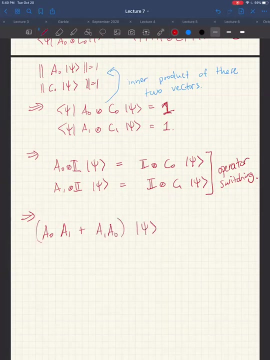 Like because- and this is the final step for this anti-commutation- I wanted to show that A zero and A one anti-commute, right. So what happens if I look at this expression? Well, I can split it like this, just by linearity: 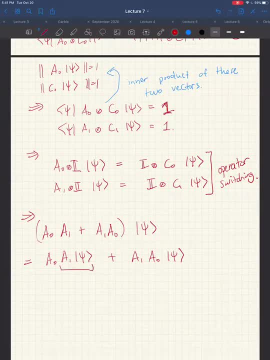 And so this thing is A one times psi. I'm going to apply operator switching, So A one times psi is the same as C one times psi. Right, Just from above. And this is A one tensor C zero times psi. But then we can just apply it one more time, right. 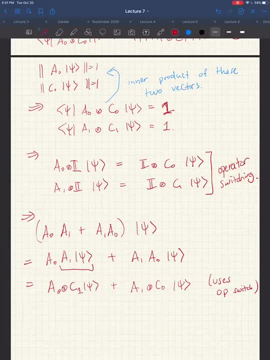 This is the same as right. We can imagine that this is identity tensor C one times A, zero psi plus right. We can just apply it one more time, because now we have an A right next to the psi. This is equal to: 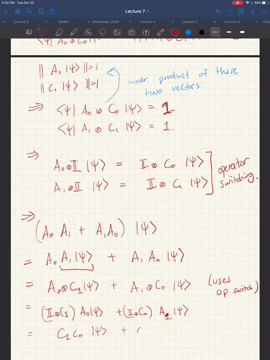 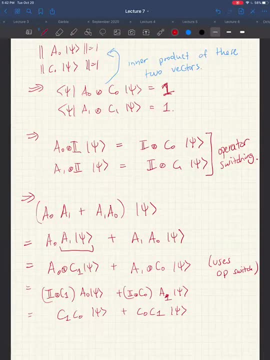 C one C zero times psi, plus C zero C one psi. And the point is that if you expand out what C one and C zero are, right, They're written in terms of these Bs. this is exactly equal to zero, And this is exactly what we wanted, because 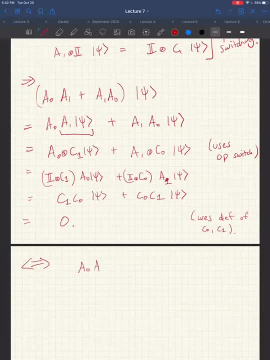 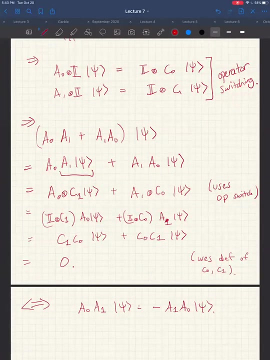 right. This is equivalent to A zero. A one times psi equals to minus A one. A zero psi Right, Which is the anti-commutation that we wanted. Can you please explain the transition where you use the auto-switching Like: why can you auto-switching? 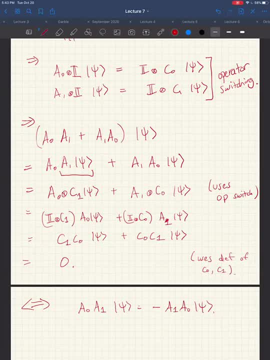 can you apply it there? You don't have it as written in your equations there, Or am I not seeing something? Oh, I guess yeah. One thing is that sometimes I've left off the identities, So whenever we see an A, technically it's. 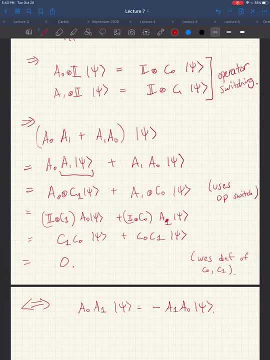 supposed to be A tensor identity. Oh, And whenever we see a, B, it should be identity tensor B or identity tensor C, And then in the next line you then have an identity before the C. Yeah, OK, It's just to save space. 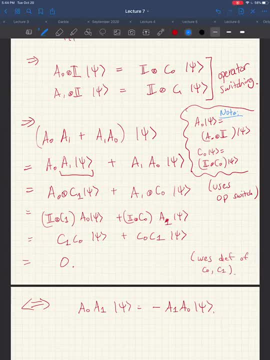 Yeah, good question. So, yeah, that might look a little mysterious, But I think it's a good idea to do that. So it's like a lot of algebra, but really, all the maneuvers that we're using, we're just using the saturation. 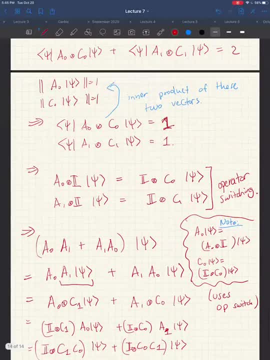 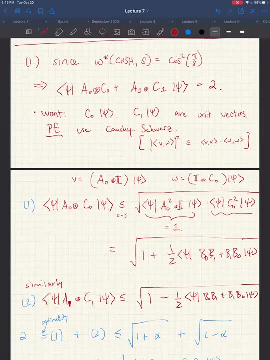 of the serosin bound a couple of times And we use the fact that A0 is an observable, so it squares the identity, And really the only non-trivial thing that was going on was this kind of clever use of Cauchy-Schwartz. 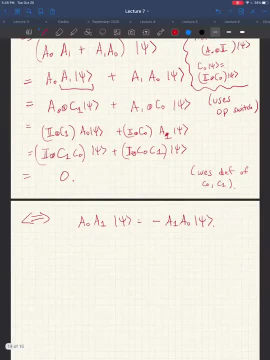 So we got the anti-commutation statement we wanted, And then of course, you could have carried all of this out for Bob's operators. So by symmetry, B0, B1, psi equals minus B1, B0, psi. 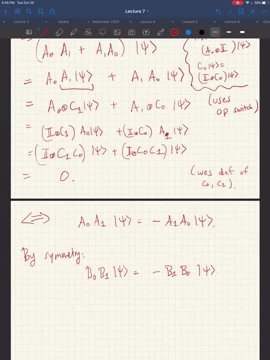 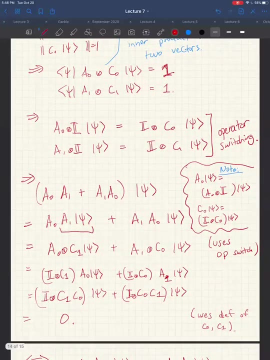 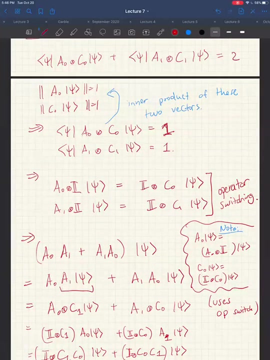 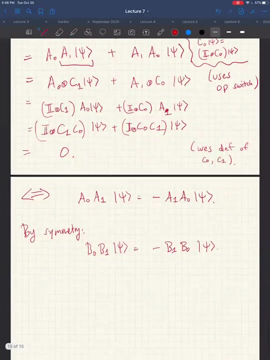 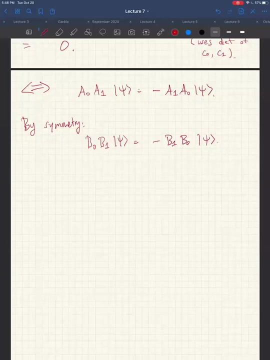 All right, All right. any other questions about the maneuvers we did or this proof? No, OK, Go ahead, Rob. OK, so that was basically most of the detailed algebra that we'll talk about Now. I'll just give an overview of these other two steps. 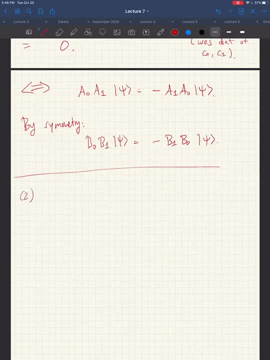 So we've got these anti-commutation steps relation. Now I claim that from this we can extract these steps, this qubit structure. I'm not going to prove this, like I think I might put this on the next problem set or something, but I'll just write what the statement is. So here's, I'll write down. 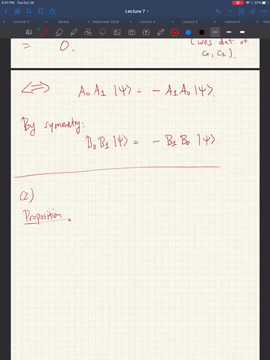 a proposition. So let's say you have- and I'll just write it like generically, like so you know, so that's abstracted away from what we have before. So let's say you have a bipartite state and you know two, you have two binary observables. 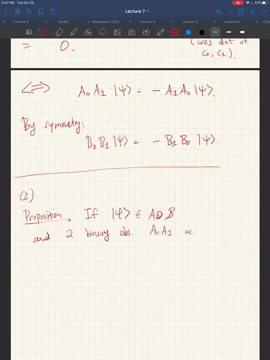 a0, a1, acting on the, a space such that a0, a1, you apply to psi is equal to minus a1, a0, apply to psi. Then there exists this isometry, local in the sense that it only acts on a. 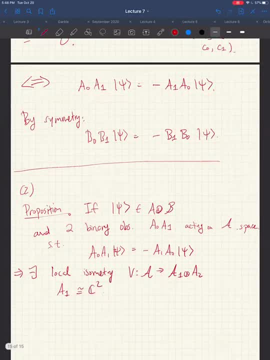 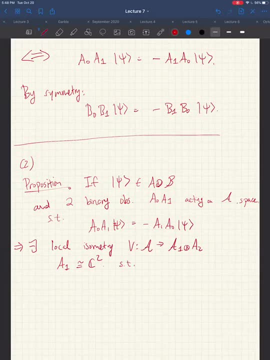 where this a1 is isomorphic to c2, such that I mean it'll just be like one half of the original theorem statement that we had. So if you had v applied to a0,, this is equal to z acting on a1,. 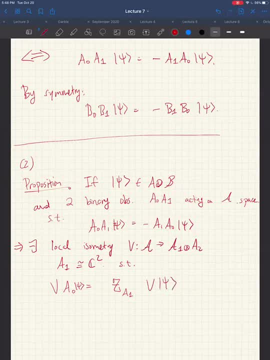 applied to v sine, and so this is just like a generic fact about anti-commuting operators. It basically if, whenever you see anti-commuting operators, morally speaking, you've located a qubit Like you can perform some basis change on which those two anti-commuting operators look like the z and x operators acting on a two dimensional space. 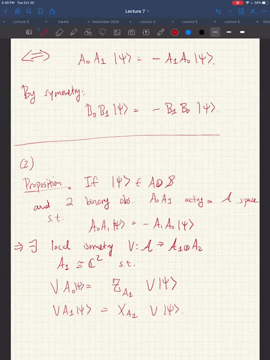 So this is just some like linear algebraic fact. Next slide, please. So actually in a lot of these like these verification performance data groups- and even when you write them in theオ, all of them tend to be very, very clear right How they operate in a square. So actually in a lot of these like these verification 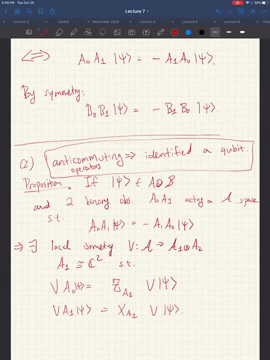 So actually in a lot of these, like these verification protocols and these verification papers, this is a very common theme that comes up. It's like, well, you're interacting with something that's completely uncharacterized. How do you know how many qubits they have? 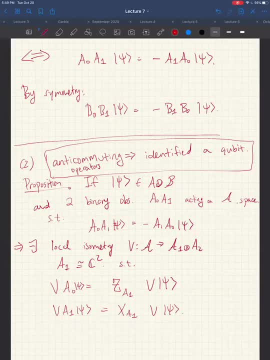 or whether they even have a qubit, And in some sense it's kind of not. It's hard to say without peering inside the box. how do you know that a qubit exists? But the point is that if you can identify, 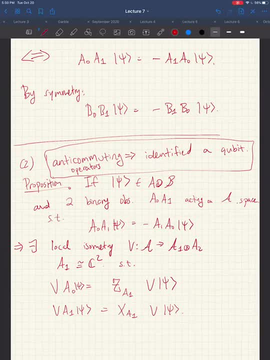 anti-commuting operators, then that defines what a qubit is Like. you don't know what basis or reference frame that this device or these two players are using. I mean, they're using an arbitrary reference frame, but you don't really care. 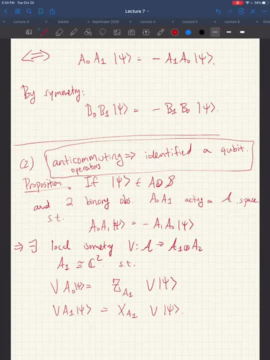 The point is that if you have two anti-commuting operators, then there's a reference frame under which those two operators look like they're just acting on a single qubit. So you just say two anti-commuting operators. that defines the qubit. 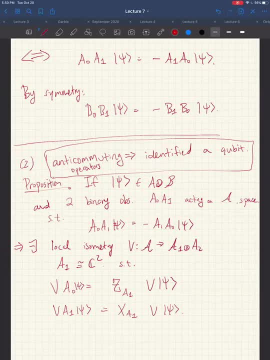 So that's a very think of. it's a simple observation, but I think a very powerful one, And so this proposition is may show up on the next problem set, And that's really the basis for a lot of these verification protocols. 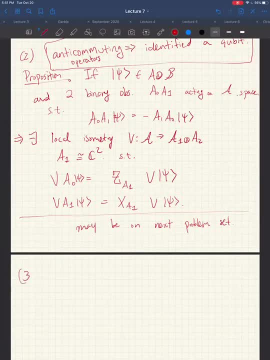 Okay, so that gives you the qubit structure, and now you have to find the EPR pair. All right, so clearly you apply this proposition, once for Alice and once for Bob, and you get these two isometries, one V, one W. 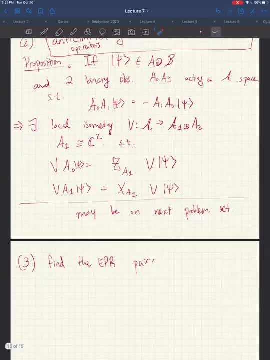 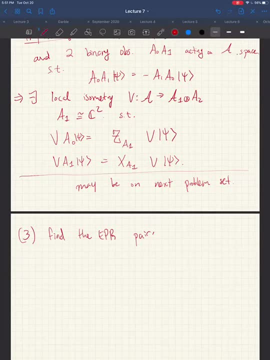 So let's see. Okay, so how do we find this EPR pair? Well, let's go back to the some of the relations we discovered. We found out that A tensor zero, A zero, tensor C zero is equal to one. 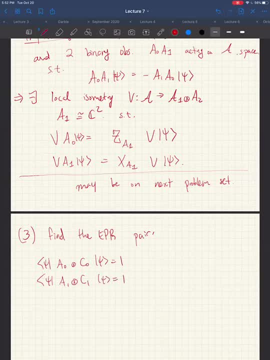 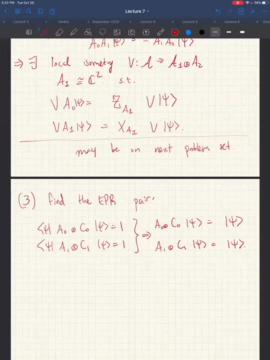 A one tensor C one is equal to one. So I mean this is just the same as this. I mean we basically prove this in the anti-commutation step. So let's apply our isometries V and W that we found to both sides. 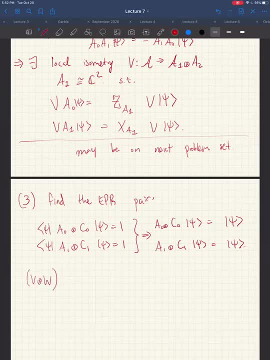 So so we apply isometries V, W, A zero, tensor C zero to Psi right, And the role of these isometries is really to just make A zero and C zero look like X or, sorry, the Z operators, right. 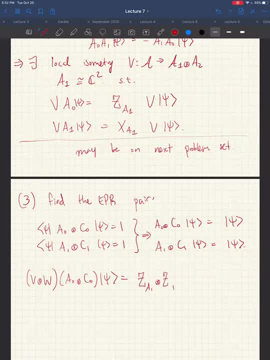 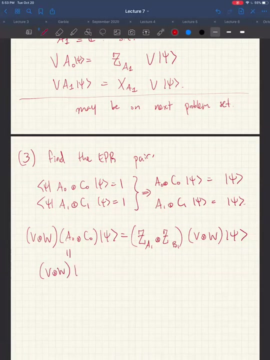 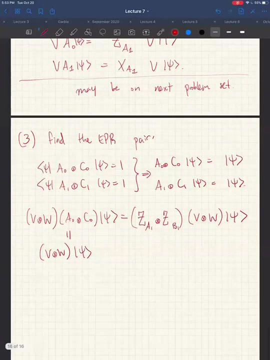 So this is Z, and Z applied to A one and V one on the on the basis change state right. But on the other hand, we know that this is the same as VW applied to Psi. So all three things are equal. 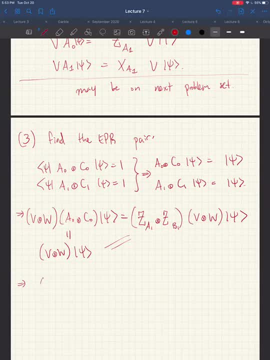 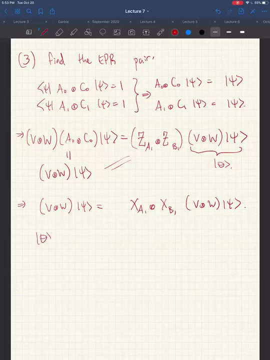 What's another thing that we know? Using the same exact reasoning, we get that V tensor W applied to Psi is equal to X, and V tensor X on V tensor W, Psi, right? So let's call this theta, right? So theta is a state on four registers, right? 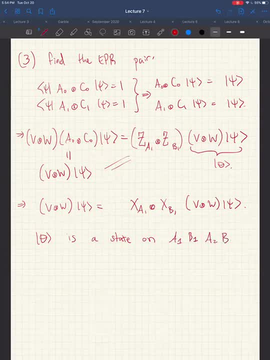 You know it's A one, B one, A two, B two. So we're just gonna put those define. So we've got the. you know let's call this U0, the secondarmazar in our recursion file. 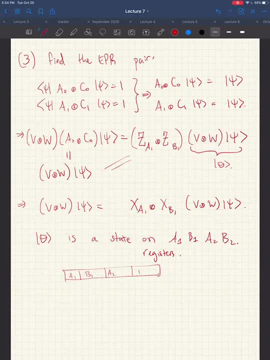 the last digit and so just to draw it like this- you know, I'm gonna reorganize the registers a bit- it says that if we apply Z and Z on these two qubits, apply X tensor X on these two qubits. 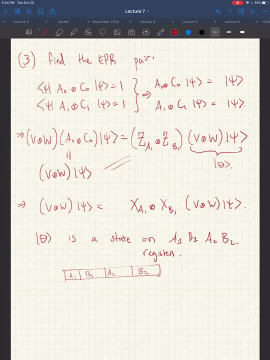 it also leaves the state unchanged. And that is the same as saying like: if you measured these two qubits in the Z basis, you get the same outcome, And if you measured in the X basis, you get the same outcome. So this should start ringing a bell. 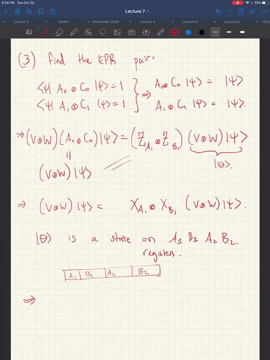 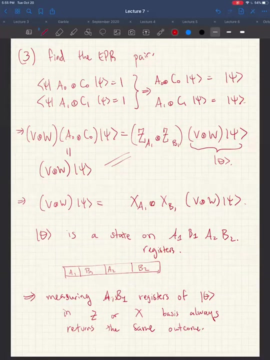 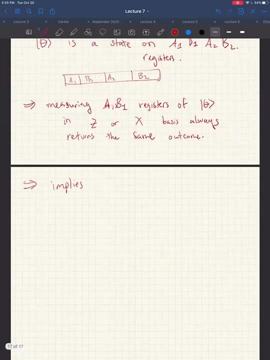 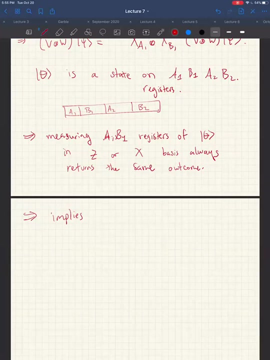 Like where have you seen this before? So what does this imply? So what does this imply? Why EPR? Exactly, It implies that in the A1 and B1 registers it has to be an EPR pair, Can't be anything else. 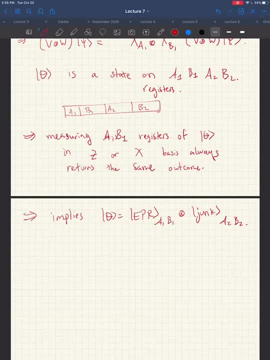 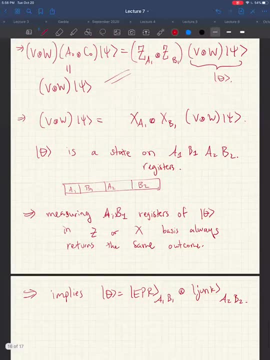 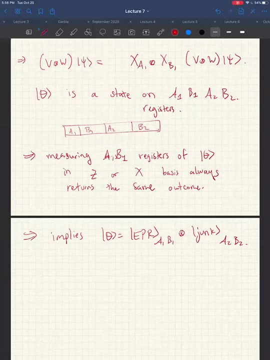 And that's it. I mean we've basically proved the rigidity statement We've. we have this local basis change. It gets us the Z and X operators and we found our extracted the EPR state And so on. 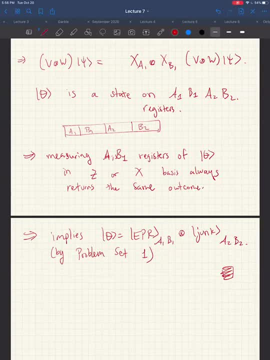 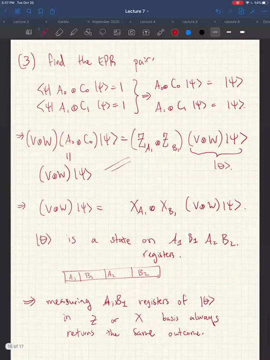 So, finally, I'd like to start with some proof. Any questions about the proof? This was heavy. Yeah, There's a lot of steps. That's interesting. I have to think about that more than I know how many people are here. I mean, you know, you know, don't worry if, if some of the details, like you know when, 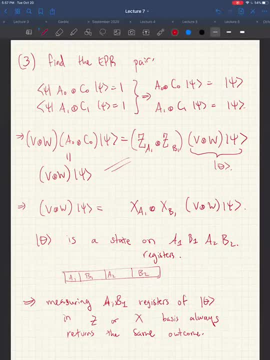 when pass you just remember that, just the main three steps. You know winning optimal means you, you can. you know that they have anti commuting measurements And from then it's sort of like that's the most important thing. then you can identify the basis change and identify with the qubits are, and so on. 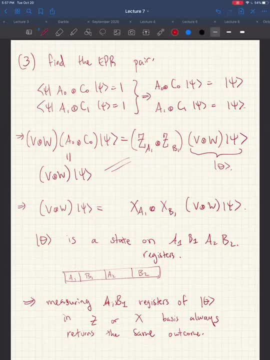 So that's, that's the thing to remember. Also, when was this proven? like how long after the? after the proof of the Bell's theorem, I guess? Oh, quite a while. So I think the earliest People reproved it a bunch of times, but I think the earliest time that it was noticed 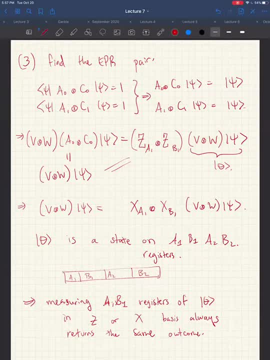 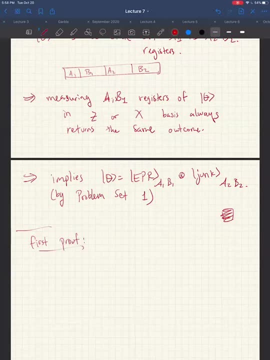 was in the late 80s. So so this is, I think, the first proof. I think my history is a little murky, but I think it's due to summers in Werner in 87. And I think Sturluson might have also realized it, but he didn't, maybe didn't bother writing. 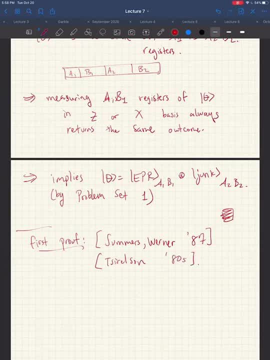 it up, Maybe sometime in the 80s, And then I think it was like rediscovered in the computer science world. Hold on, Who was it? I don't know Something like that. I don't know, I don't know. 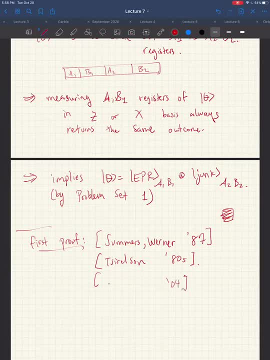 I think it was some time before the end of the 20th century. I think it was sometime like 2004.. Forget who. I know that Andy was on the paper. So it was proved in a bunch of times separately by different people. 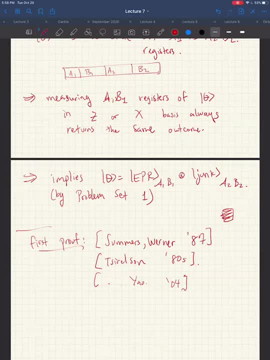 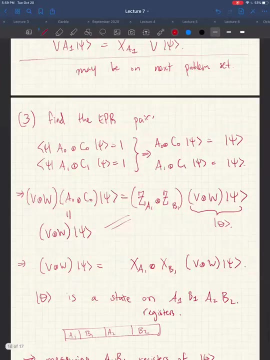 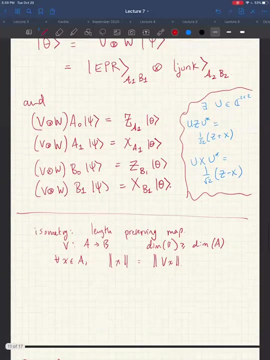 Okay. so the last thing I wanted to mention- Okay thing I wanted to mention- was: you know, this proof, yeah, it's heavy, has a lot of steps, But you know there's one big thing that you should be dissatisfied about. 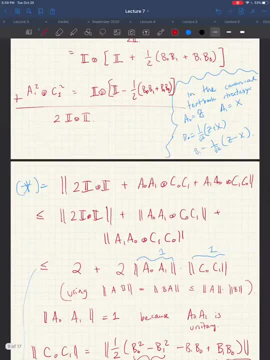 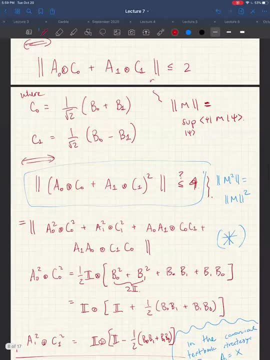 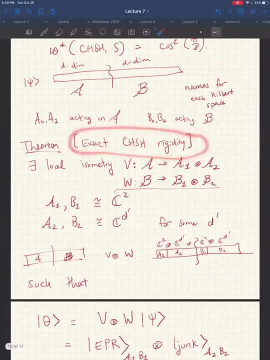 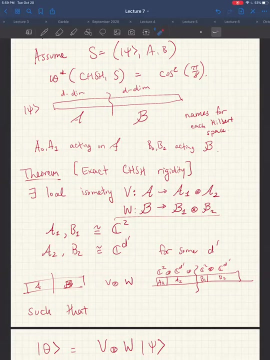 other than the fact that it's long. Yeah, so you might be dissatisfied with the fact that we only proved exact rigidity. But how do you, you know how often- can someone give you a strategy that wins with exactly a certain probability? right, Like, how do you even test that a strategy has, you know, co-squared? 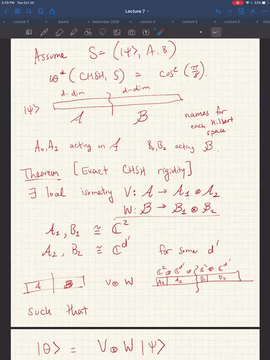 pi over eight success probability. How do you even test that a strategy has, you know success probability? How do you even test that a strategy has, you know, co-squared pi over eight success probability? I mean, you can right. You're just playing this game multiple times. 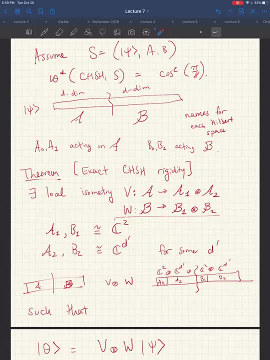 and you're just trying to estimate how often they win And you can only know that they win with, say, you know, 84% or something right. So suppose that you know that they're winning with probability optimal minus epsilon? What can you say about their strategy? 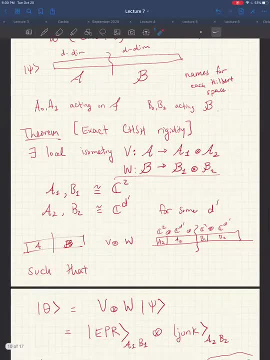 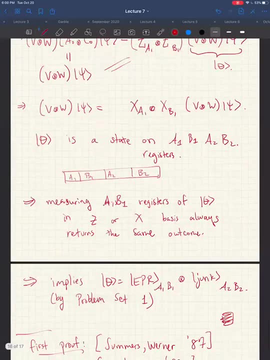 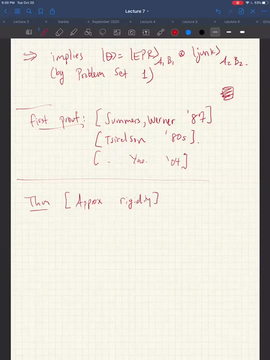 And it turns out that you can basically say the exact same things except all of you. instead of equality, you just have approximations. So what's true is approximate rigidity. So you say, suppose that the value of your strategy is, at most, you know. 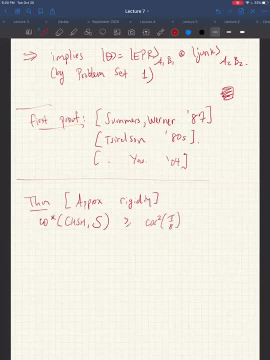 the close squared pi over eight minus epsilon. for some epsilon, then it applies that this theta, like there's still these local isometries, it's going to be not exactly but square root of epsilon close to this EPR And all of your operators. 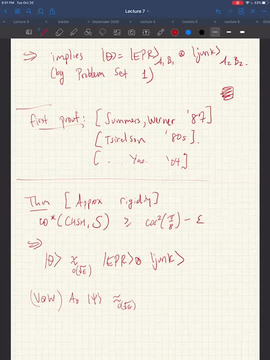 approximately look like the. you know the Z and X operators, So it's really the same thing, but you just put square root epsilons everywhere, And this is really the thing that's most useful in practice, because of course, you can never know. 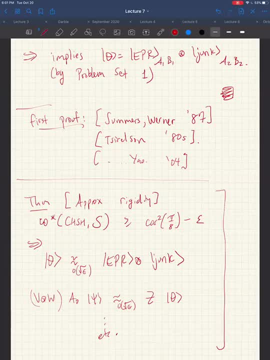 that they went perfectly, but that they went close enough to perfect, And it's the same proof. You're just keeping track of all the epsilons. Is this known to be a tight trade off? Or, Yeah, the squared epsilon is unnecessary.